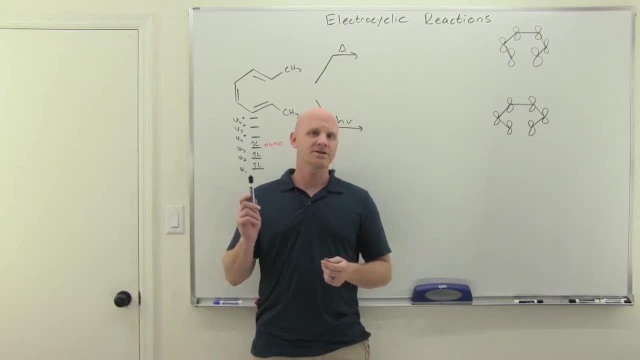 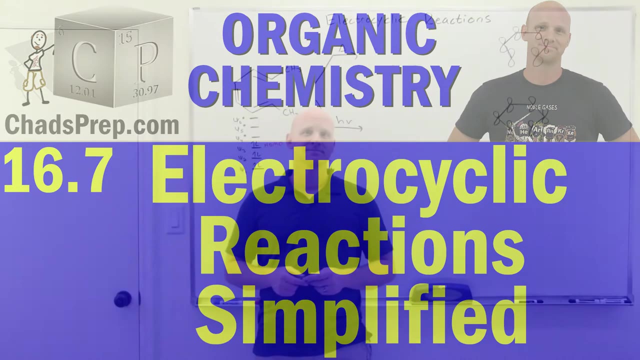 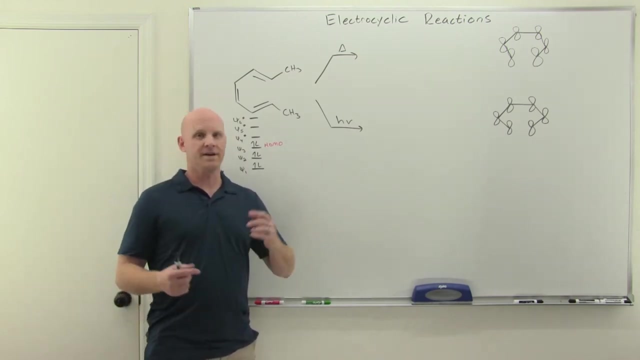 But by the end of this lesson I promise you're going to have a much better handle on your electrocyclic reactions. All right, so electrocyclic reactions. So typically electrocyclic reactions are either going to be a ring closure or a ring opening, And it turns out they're just reversible reactions. In fact, there's typically an equilibrium established And, depending on the size of your ring and if it has ring strain, things of this sort, those kind of considerations will determine which will be favored: either the open chain or the ring. 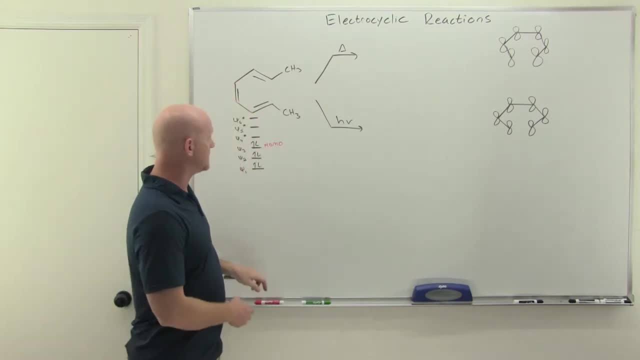 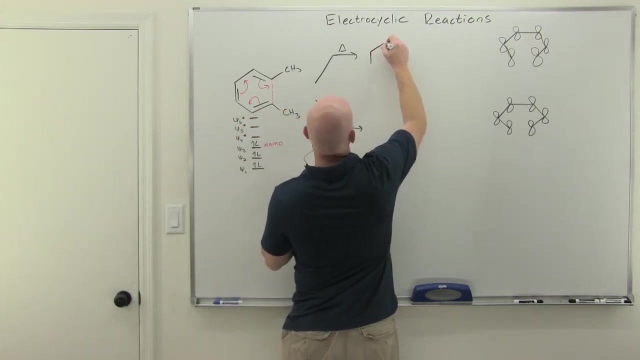 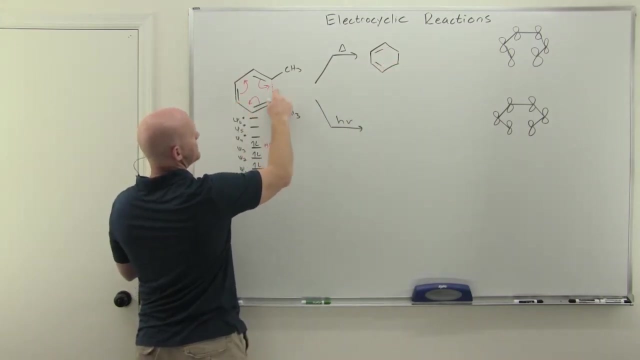 Cool. So in this first example here we're going to look at a ring closure specifically, And in this case we're going to have the cyclic movement of pi electrons to form a ring, And so in this case we can see that we're going to form a six-membered ring, And in this case we'll still have pi electrons here and here And then we'll get the new sigma bond here. 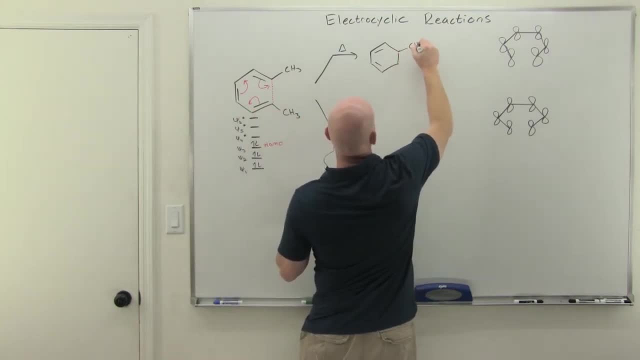 So we're going to have something like this, And the problem we're going to have is with stereochemistry here. So we've got a methyl group here and a methyl group here, And the truth is so far, based on what we've shown, there's no difference with our photochemical conditions as well. 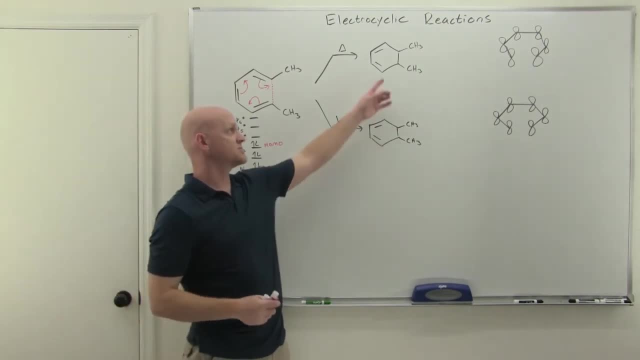 So we've got thermal and photochemical. What is going to be different, though, is the stereochemistry. I'm going to erase these straight-line bonds and draw in wedges and dashes in a little bit, and we'll see the difference. 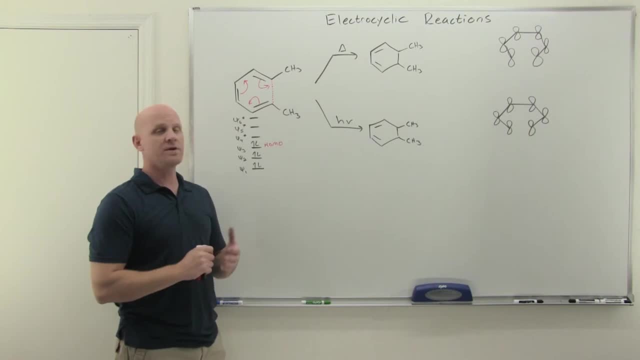 Now, how we predict this, we'll see here with orbital symmetry and things of this sort. So now one thing to note here is: this is not like a cycloaddition, where we have two reactants. We just have one reactant. 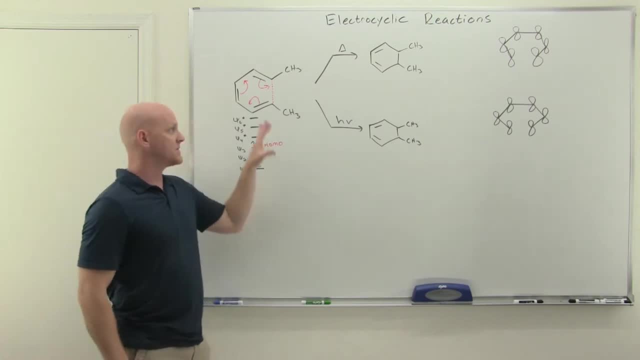 And so we don't have to like draw the HOMO of one and the LUMO of the other With an electrocyclic reaction. you're just going to involve the highest occupied molecular orbital of your only reactant, And so it's all about the HOMO, not about the LUMO. 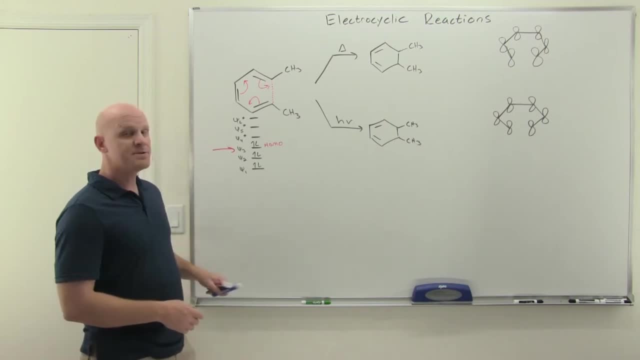 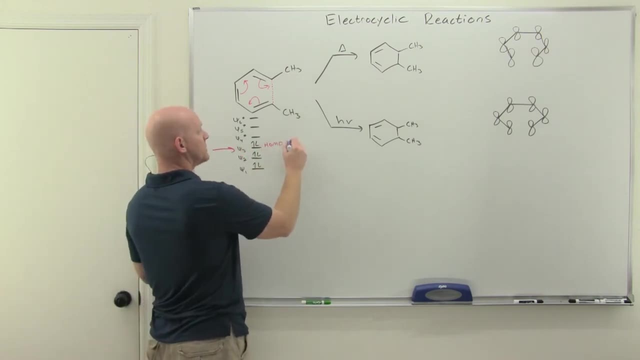 All right, In this case you're going to want to figure out your symmetry there as well, whether it's symmetric or anti-symmetric. And notice again: psi 1 is always symmetric, then psi 2 is anti-symmetric and psi 3- here an odd number- will also be symmetric. 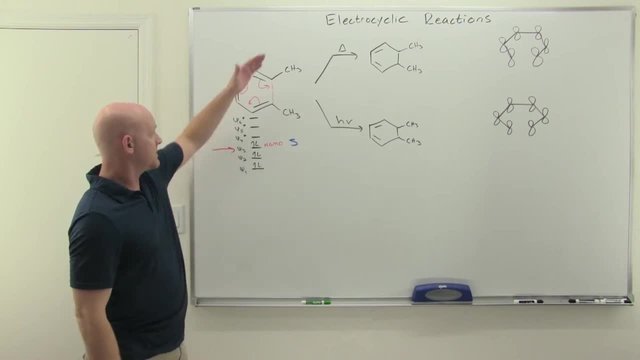 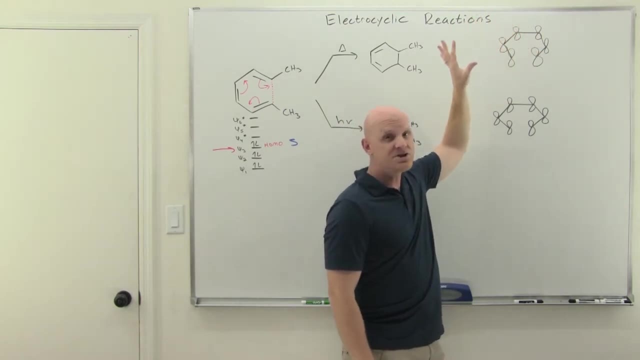 And that will be super helpful. And so, under thermal conditions, here we've got psi 3,, which is symmetric, as our highest occupied molecular orbital, And so we're going to draw him up here Now, just like with the cycloadditions, though again you're probably going to be on the hook for having to draw the entire psi 3 on there. 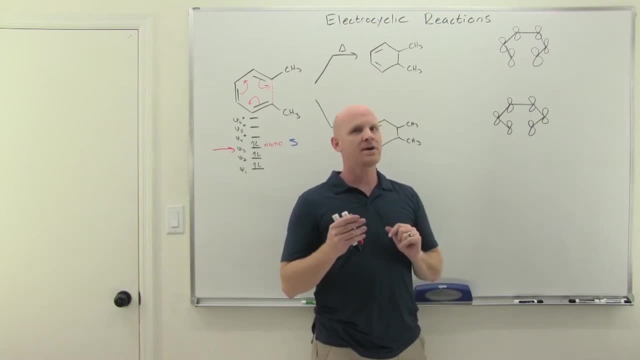 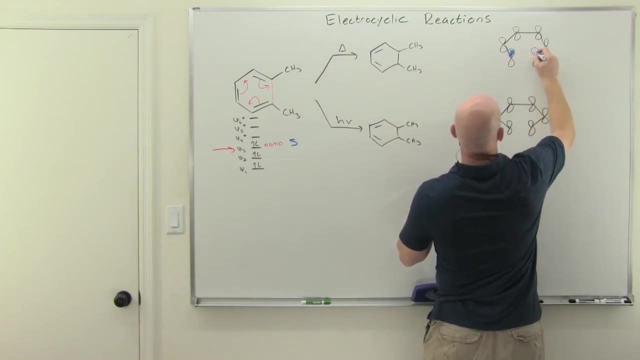 However, in terms of predicting stereochemistry, the only part that really matters is the ends And, knowing that it's symmetric, I'm only going to draw the ends in here. And, being symmetric, they just matter, They match. Now, if you got the study guide handy, I drew the entire psi 3 molecular orbital there so you could see it. 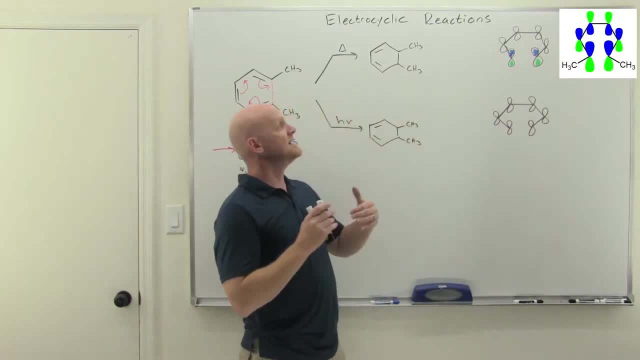 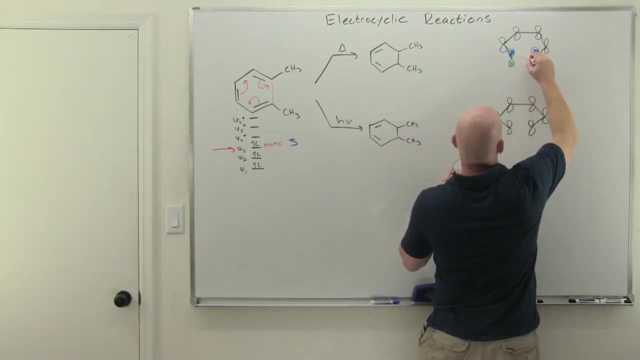 But again, the only part that I really need for predicting the product in the stereochemistry product is just those ends. And so it turns out what's going to happen when you form a new bond right across the middle. here is it turns out that the molecular orbital at the ends is going to rotate in one way, shape or form. 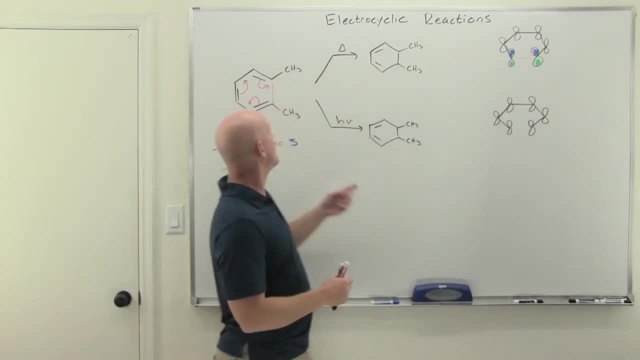 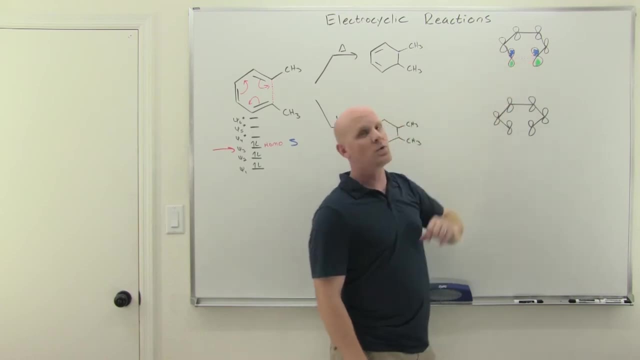 And when it rotates we're trying to get constructive overlap to create that new sigma bond we're forming right there that ends up in the product right there, And so we're actually going to rotate the ends of the molecular orbital here in one way, shape or form, to cause that to happen. 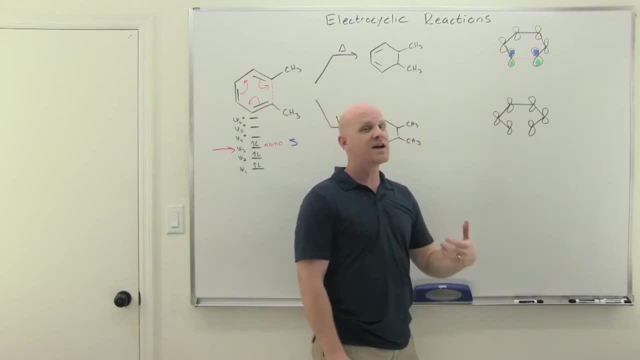 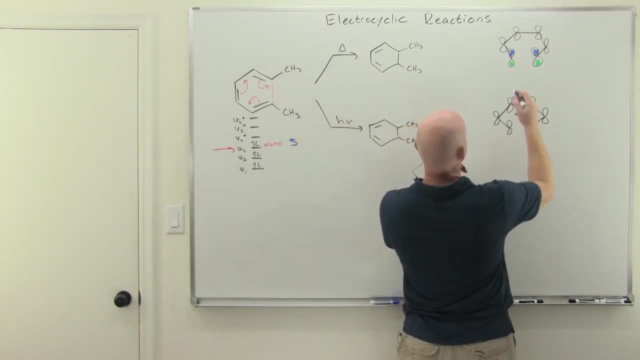 Now what we're going to do here is rotate this either clockwise or counterclockwise on the left-hand side and then just match it up on the right-hand side so that we get constructive overlap. And what I want to have happen here is we want to turn these. 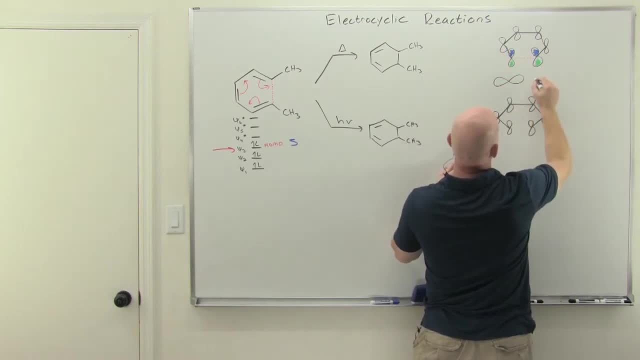 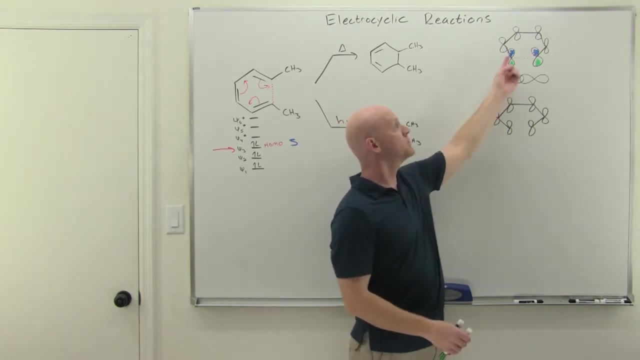 And let's say I rotate this one clockwise in such a way, And then this one I'd have to rotate either clockwise or counterclockwise And I'm going to try and get constructive overlap where they've rotated, In this case either both blue, as I've drawn it, or both green. 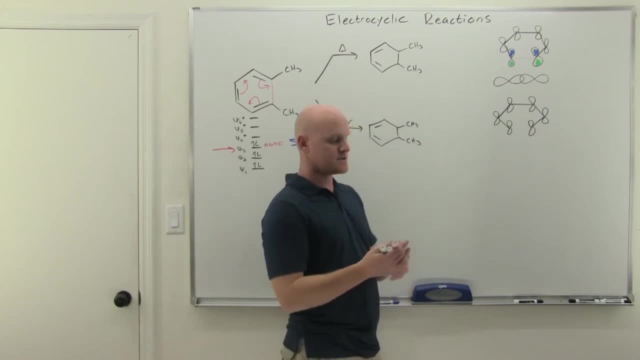 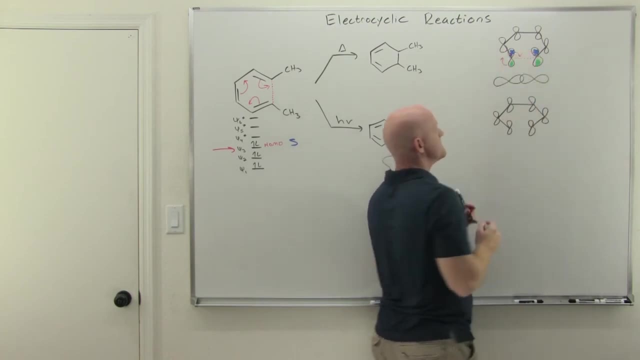 And it could be either way, which is why we typically end up with two options for how to accomplish this, And so, in this case, let's just say I choose to rotate this end of the molecular orbital clockwise, so that it would put the blue region into the middle. 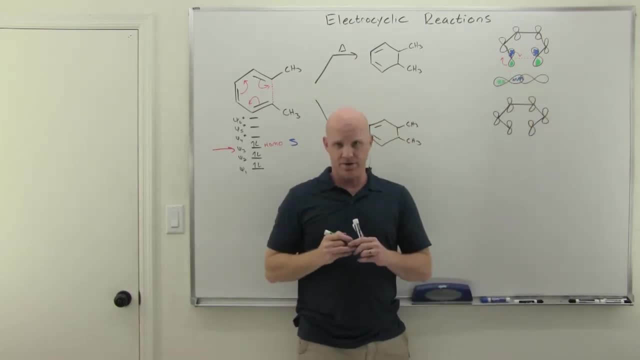 And again, I could have chosen counterclockwise, which would put the green region into the middle. So either way works. It's arbitrary. But once you've chosen one side, the other side has to rotate in such a way that it puts the same phase in the middle there. 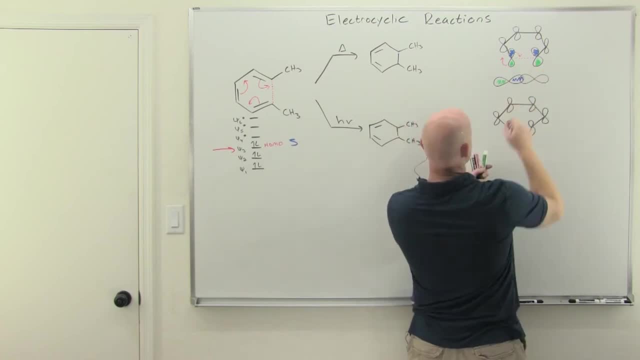 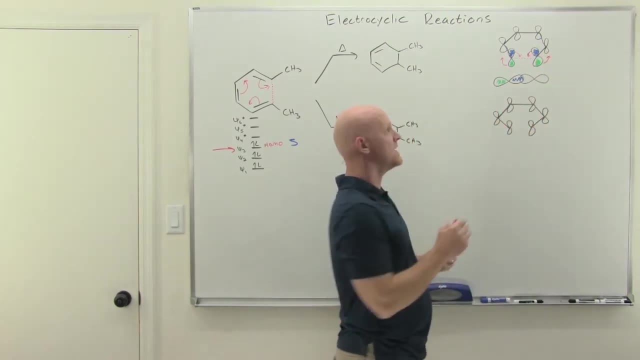 And so in this case, if the blue is in the middle, then I need to rotate this one in such a way that the blue ends up in the middle, And in this case I can see that instead of rotating it clockwise, it'll be counterclockwise instead. 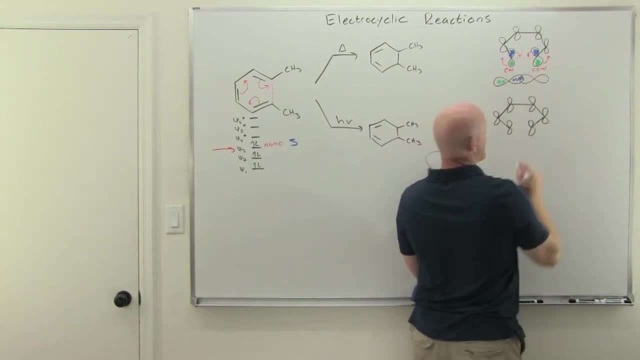 So the one on the left I chose clockwise. the other one ends up counterclockwise. Now, had I chose the one on the left to be counterclockwise, this one would have ended up clockwise and they both would put the green. 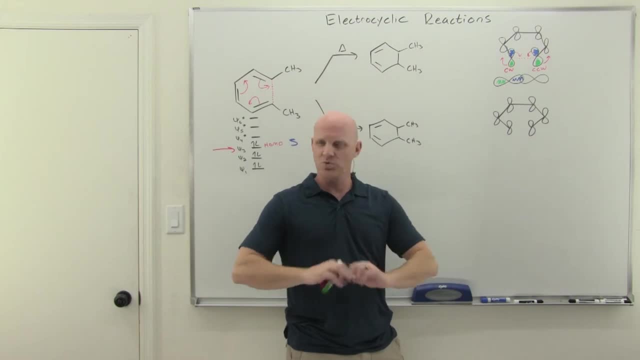 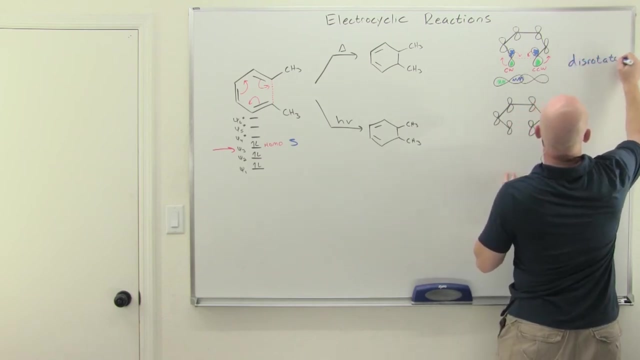 The green portion is in the middle. As long as it's in phase and constructive overlap in the middle, great. That's exactly what we need to accomplish. But we have a name for this. When one side is clockwise and the other side is counterclockwise, when they're opposites, we call this disrotatory. 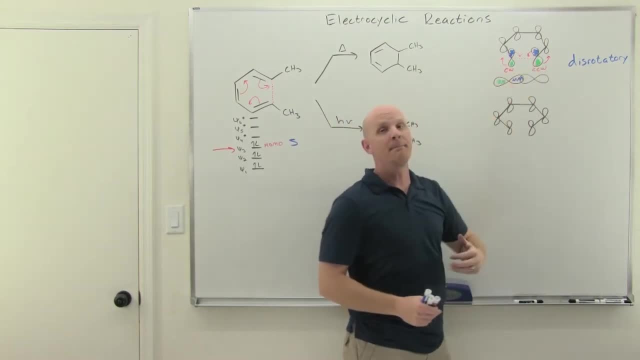 And you can see here that if the ends of your molecular orbital match, so to speak, well then it's going to have to be disrotatory. So the converse of this is what we call conrotatory. So disrotatory is like this: 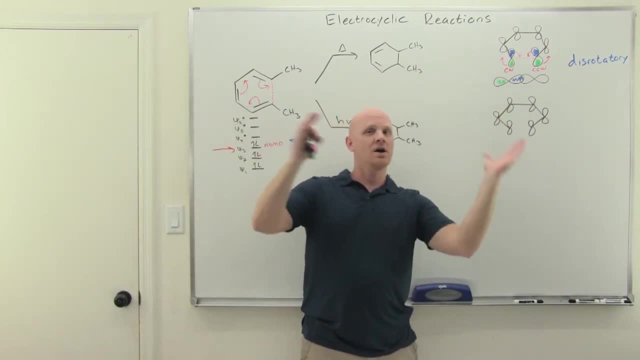 So kind of like how a lot of British windshield wipers wipe So. conrotatory, on the other hand, is when they both go clockwise or both go counterclockwise, like a lot of American windshield wipers work. So, and if disrotatory here is, we figured this out. that's what we mean really to say is that disrotatory is allowed. 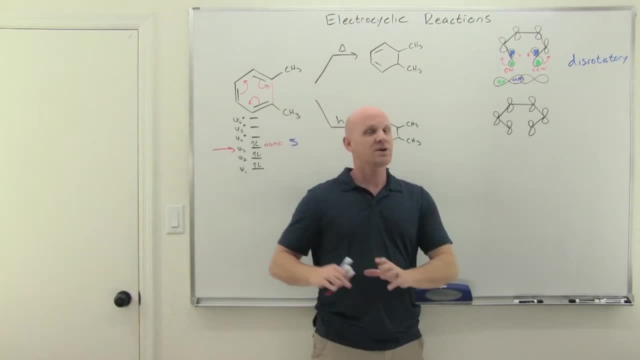 which then means that conrotatory is forbidden. So kind of similar to what we saw at the cycloadditions, where we said: well, if superfacial superfacial is allowed, well then superfacial anterofacial is forbidden under certain conditions. 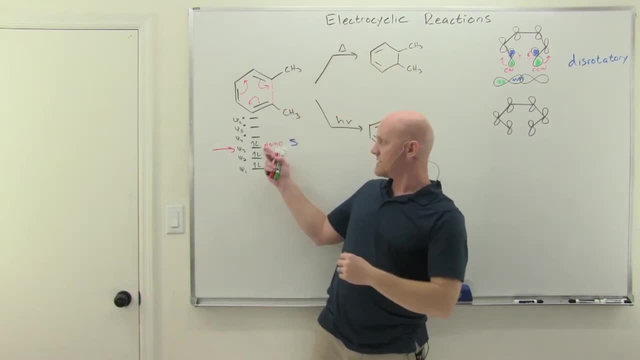 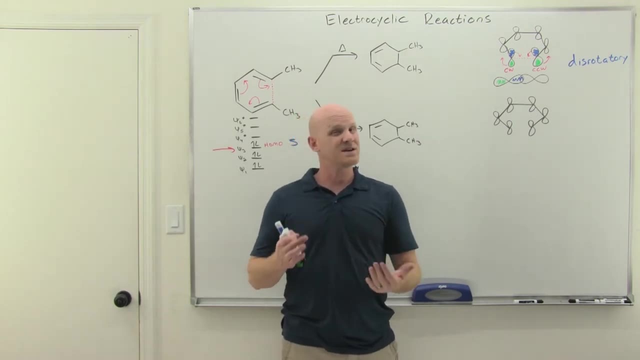 Well, in this case, under thermal conditions, where we're using psi three, which is the homo, So disrotatory is allowed and conrotatory would be forbidden. And once again, because something is forbidden doesn't mean it doesn't happen. 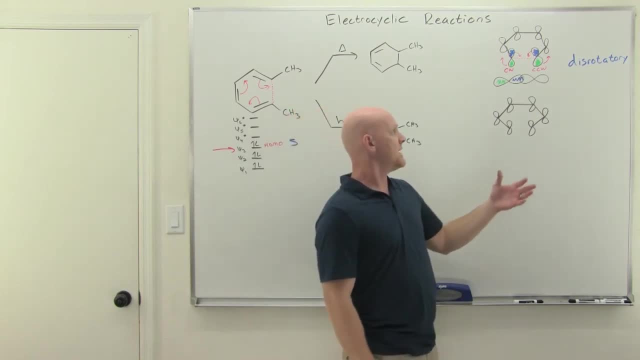 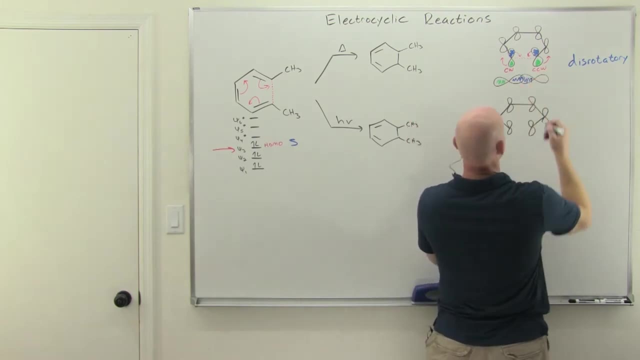 It just means it's probably not the major product, All right. So in this case, with rotating this one counterclockwise, it puts the blue region in the middle. We get that constructive overlap and life is good. Now one thing to note, if you notice when I rotated, 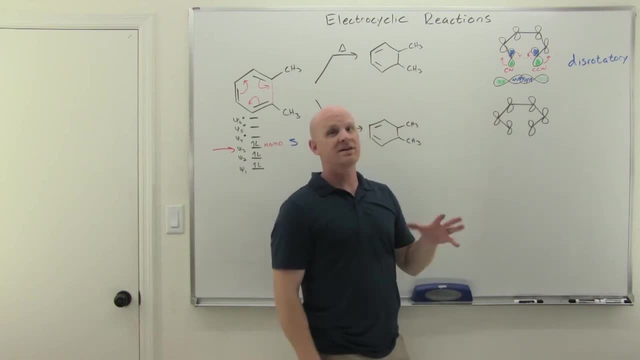 I showed two arrows For both lobes to kind of show the overall rotation clockwise, because a lot of students do this and they would just draw that one arrow and they say it rotates to the right. Well, you got to be careful what you define as right and left, because this one looks like it's going to the right. 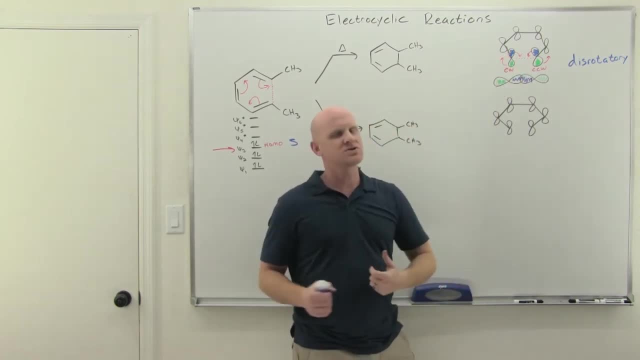 This one looks like it's going up to the left. You know so. right and left aren't the most descriptive terms, but clockwise and counterclockwise probably what you want to use here, And when I see that one's clockwise, one's counterclockwise, that's what disrotatory means. 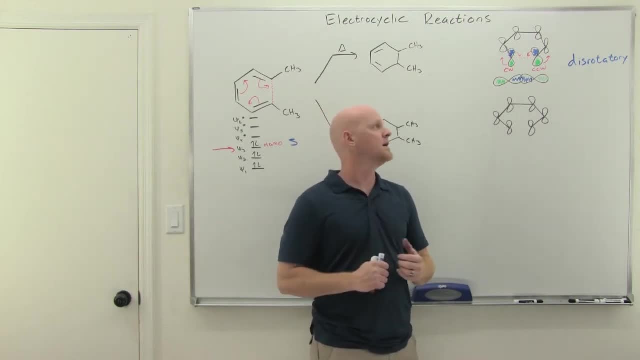 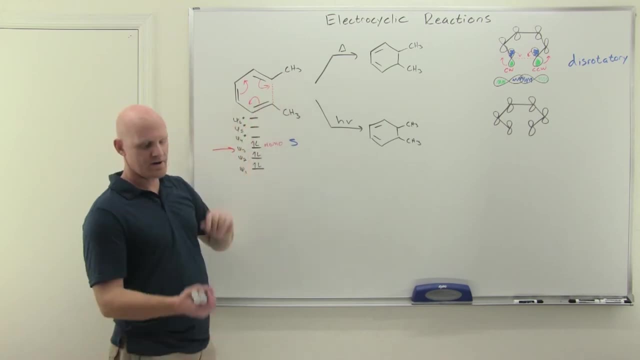 And again, if they were both clockwise or both counterclockwise, that's what conrotatory would mean. Now, the reason this is important is because now we're going to use it to predict stereochemistry, And so look at your methyl groups here. 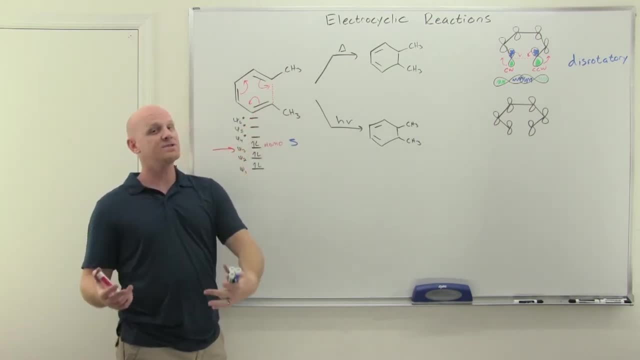 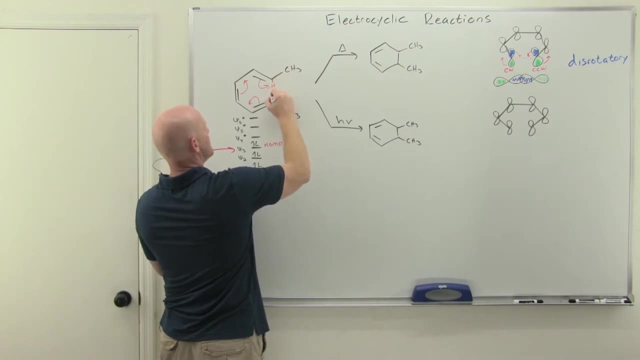 And, just like we did with Diels-Alder, we're going to define them as being either out or in, And to kind of help us figure that out, I'm going to draw in the relevant hydrogens here. There's a hydrogen right there and a hydrogen right there. 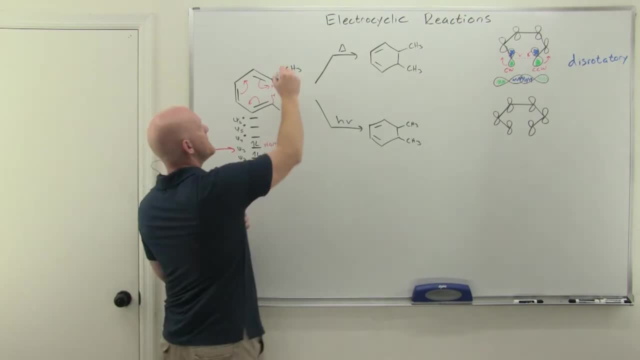 And so if you had to define the methyl and the hydrogen- one is in and one is out- well, the methyl group would definitely be the out position in both cases. So they are both out in this case. That's the main point here. 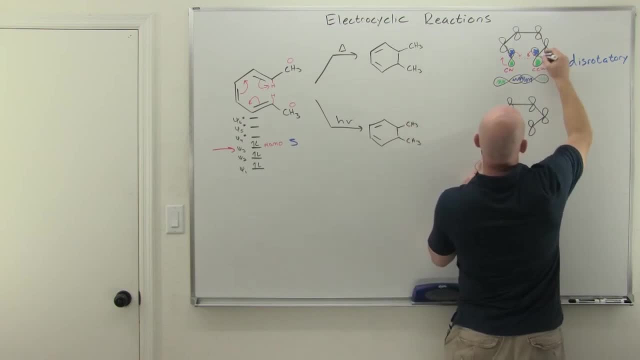 So what that would mean if you're drawing them on the molecular orbital picture here. so this is just plain 1, 1, 3, 5 hexatriene, but we've got these extra methyl groups. but they both point out. 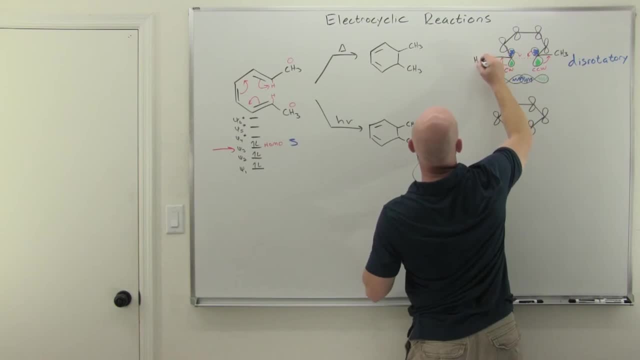 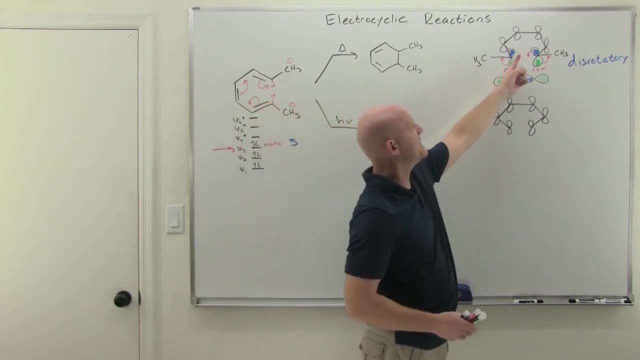 So one's there and then one points out on the other side, Neither one pointed in toward that region. That's where the hydrogens pointed. Well, what's nice is when you look at your rotation- and again, this is why I draw two arrows- 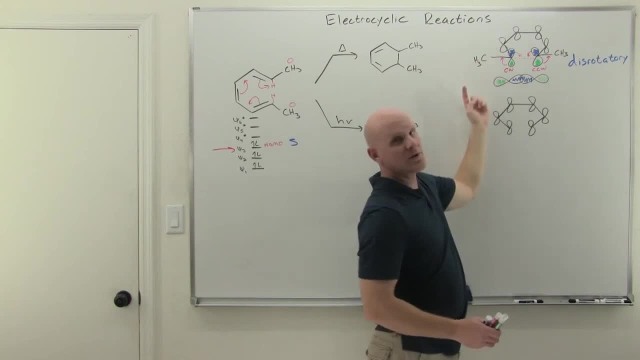 now I can see on this side that this methyl group is going to get pushed up, And when it gets pushed up, that means it's going to be a wedged bond on the product, Whereas this one over here also gets pushed up, which means it's also going to be a wedged bond on the product. 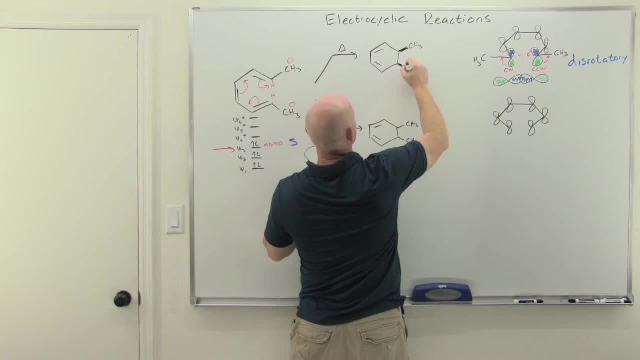 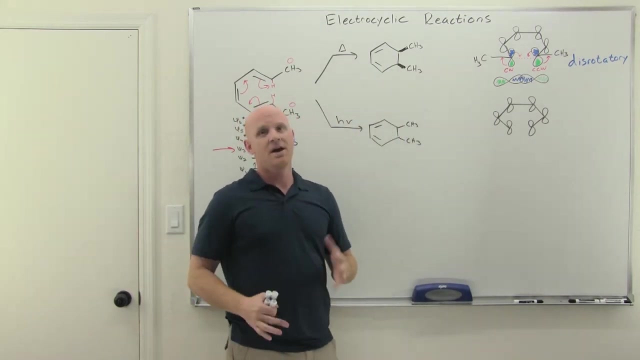 So I get two wedged bonds here, and these end up cis to each other. All right now. had we chose to go counterclockwise here and clockwise over here, well then these would have both ended up dashed bonds, and you get the opposite version of this. 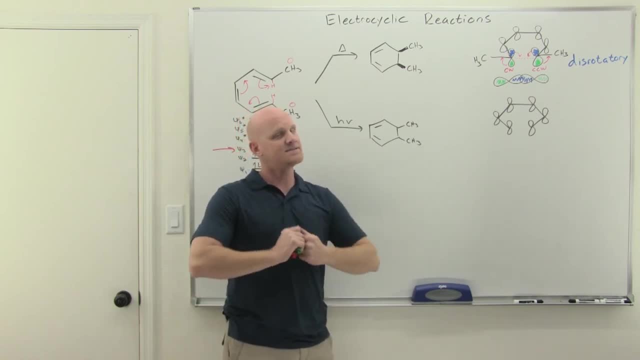 Well, in this case this is a meso compound. so whether they're both wedges or both dashes, it's the same meso compound. But had it not been a meso, it would have drawn out two products, All right, so this is kind of the deal. 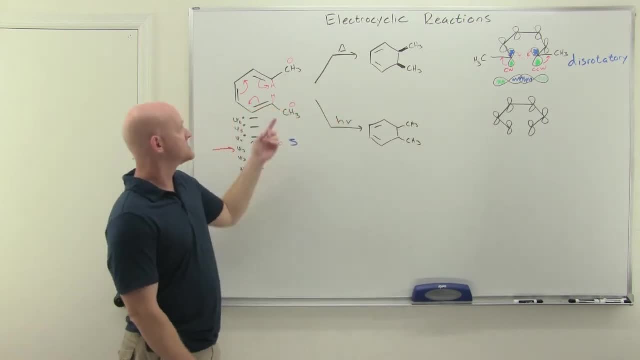 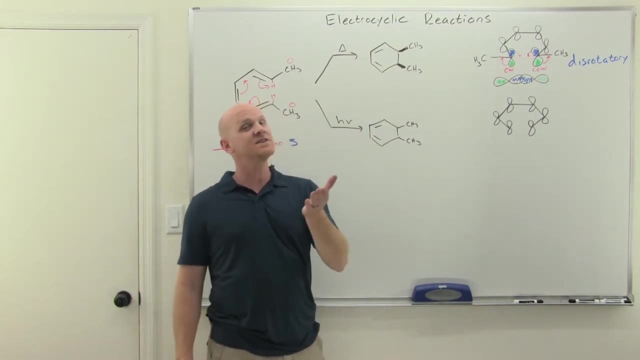 and this is kind of nice and convenient as well, because if you look here, so here they both pointed out and they end up cis. Now, this is not a cycloaddition, but that's what Diels-Alder did as well. 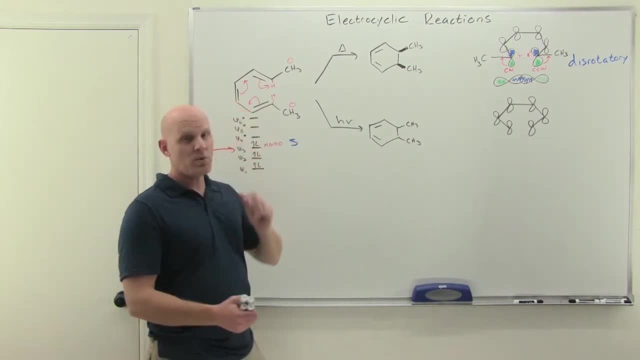 And, if you recall, Diels-Alder dealt with six pi electrons in motion and here we've got six pi electrons in motion And it turns out we can make a broader principle here that this is what we typically see for four n plus two pi electrons. 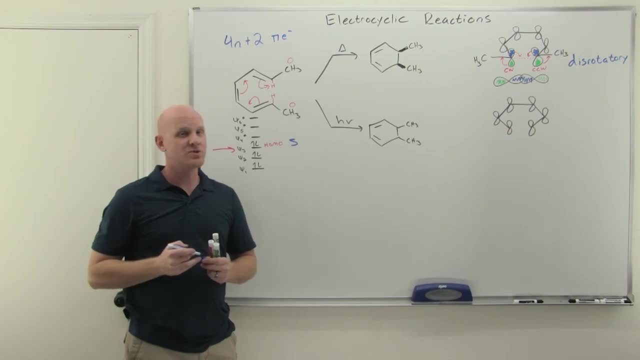 moving in the transition state. We've got to define them. moving in the transition state, as we'll see in a minute, It's not just the number of pi electrons necessarily in the system, but the number moving in the transition state. Again, that'll be important in a minute. 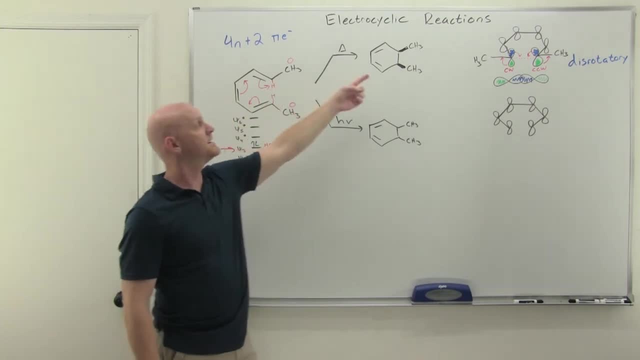 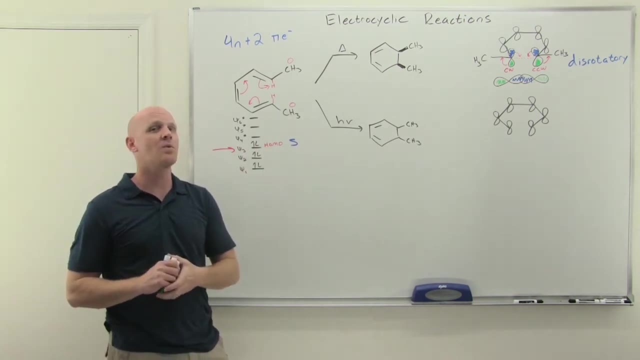 And we see here that if they're both out or both in they're going to end up cis on the product, and had one been out and one been in, they'd be trans in the product under thermal conditions, just like we saw with Diels-Alder. 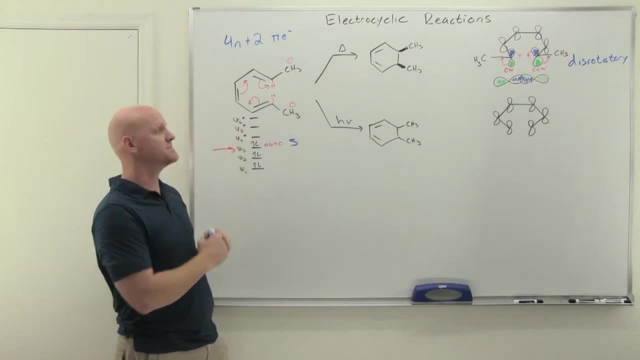 So it's convenient to kind of relate this back to Diels-Alder, even though this is not a cycloaddition but an electrocyclic, because as far as stereochemistry is concerned, it's totally analogous. Now, if we look at what happens with photochemical conditions, 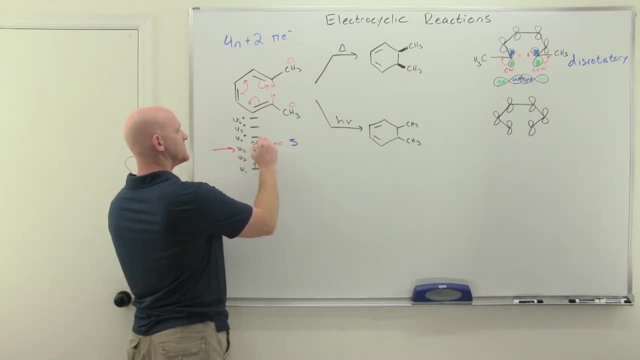 well, again, with photochemical conditions, we are going to promote an electron here from psi three to psi four. And if all of a sudden we promote an electron up there, well then we can't call psi three the highest occupied molecular orbital anymore. 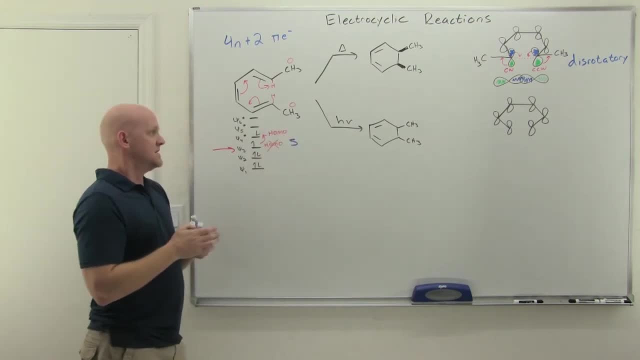 It would now be psi four. So under photochemical conditions we now have psi four as the highest occupied molecular orbital, and that is anti-symmetric, not symmetric, And so when we go to draw this out again, so now being anti-symmetric, 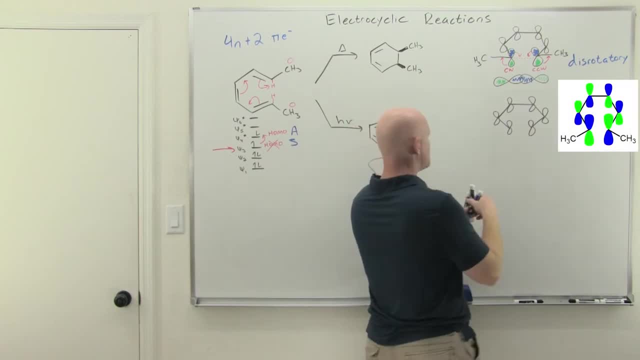 and again. I could draw the whole thing in and on your study guide. it's there, But again, the only part that really matters to me are the ends And, being anti-symmetric, they don't match. Now, before we even show the rotations, 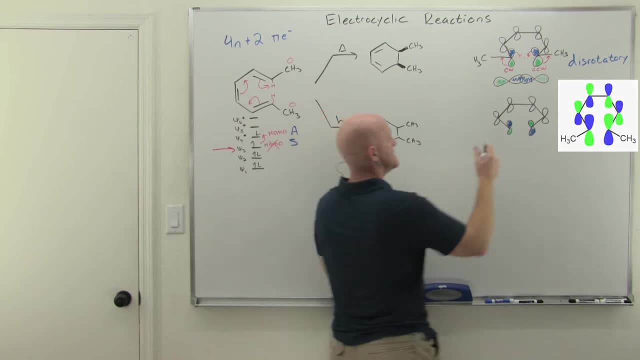 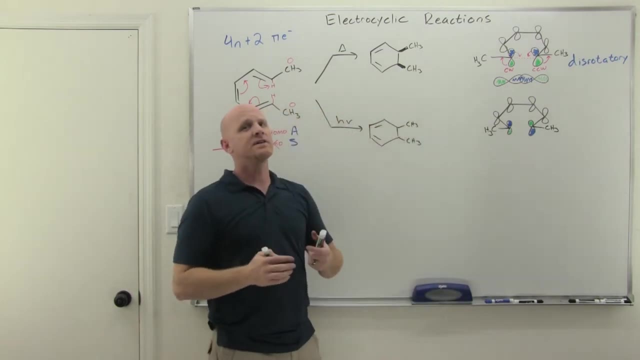 I'm going to preemptively draw in our methyl groups, which again point both out. So we'll put one out over the other, One out over here, One out over here. But now, once again, we want to rotate the ends of the molecular orbital here. 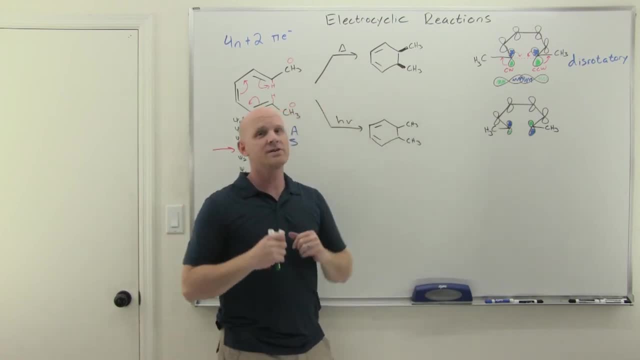 this end and this end, either clockwise or counterclockwise, to lead to constructive overlap in the middle. And again, I, like you know, usually I'm pretty systematic about this and I just pick the one on the left first. 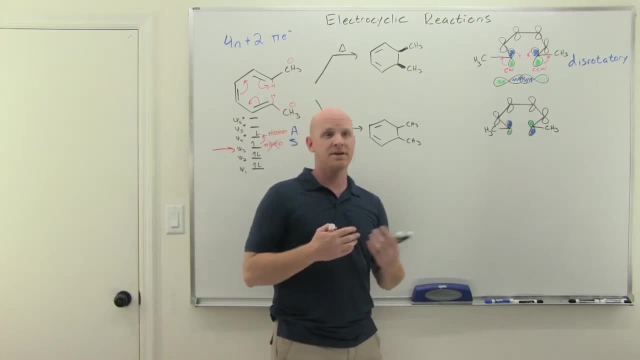 and I make it go clockwise almost every time. But you could pick the one on the right first or you could pick the one on the left to go counterclockwise. It's really arbitrary: the first one. So this is what I do. 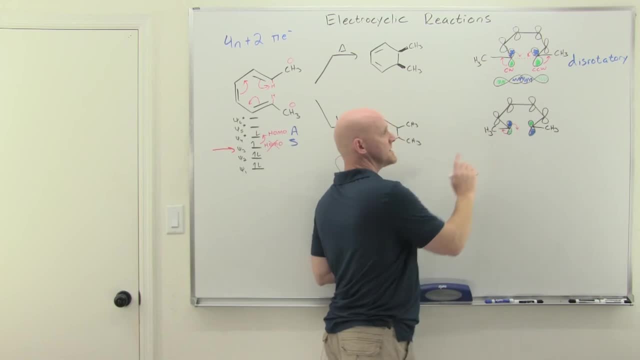 One on the left, going clockwise, And I can see that that methyl group is going to get forced up. It's going to be a wedge in the product. That's the first part, And so in this case, if you notice, if I rotate this around like so, 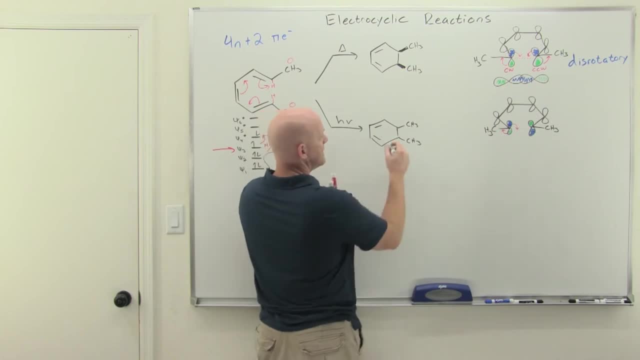 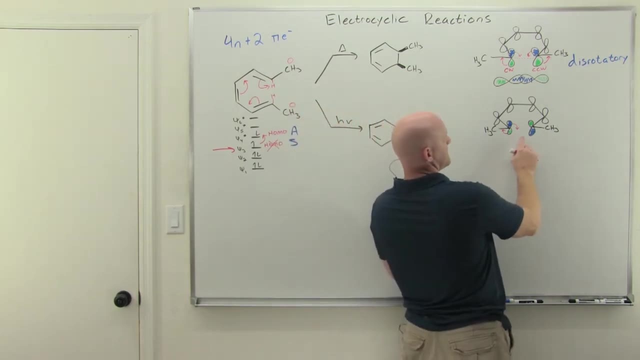 that one right, that methyl group right there is that methyl group right there, And so I can see that it's possible for it to get a wedged position. So, but on the other side here I can see that if the blue region 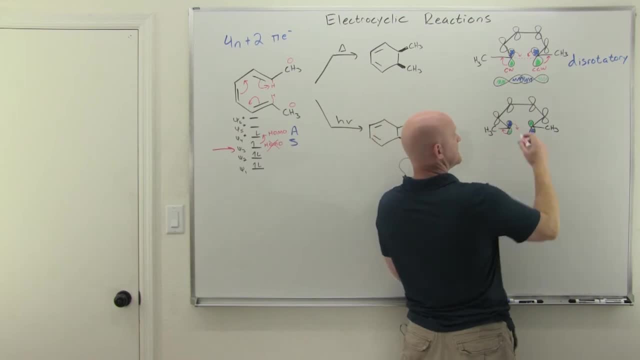 is going to be out facing the middle where we're forming the new sigma bond, then to get the blue region on this one facing that same place, so I'll need to rotate this one also clockwise. so now they're both clockwise, Which means this is not disrotatory. 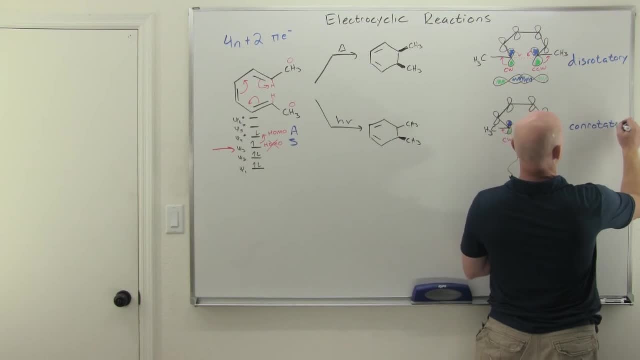 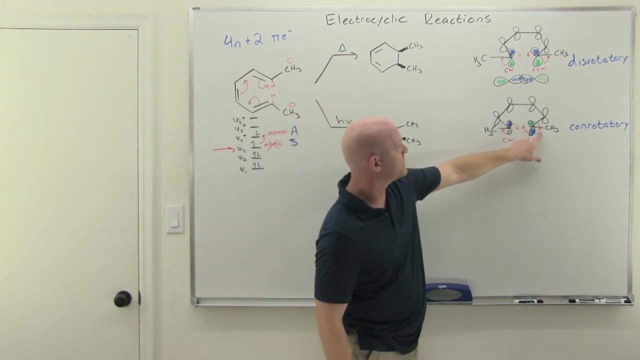 this is conrotatory, And so now it's conrotatory that would be allowed and disrotatory that would be forbidden. I can also see where that other methyl group's going, That other methyl group on the other side. notice again. this is why I make sure to draw both arrows. 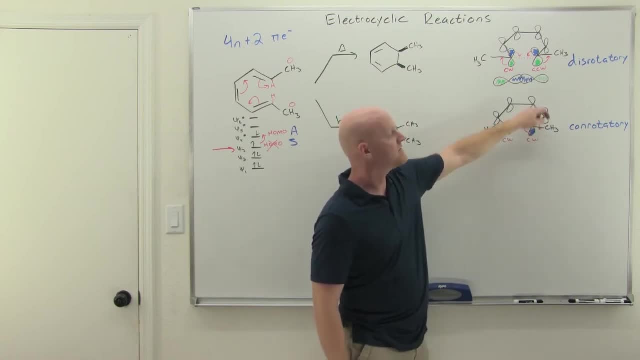 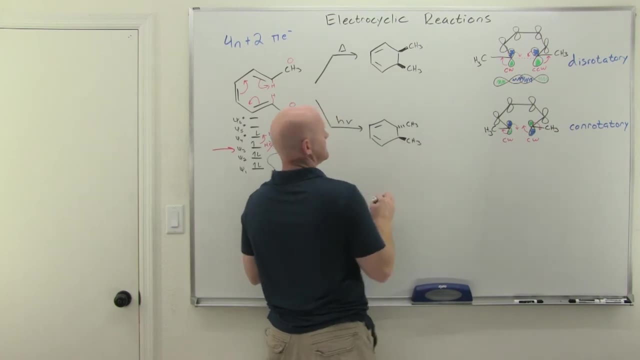 to show the complete circular motion. I can see it's getting forced down and it's going to be a dashed bond, So in this case this is not a meso compound. Now there's no plane of symmetry down the middle, And so I get both versions. 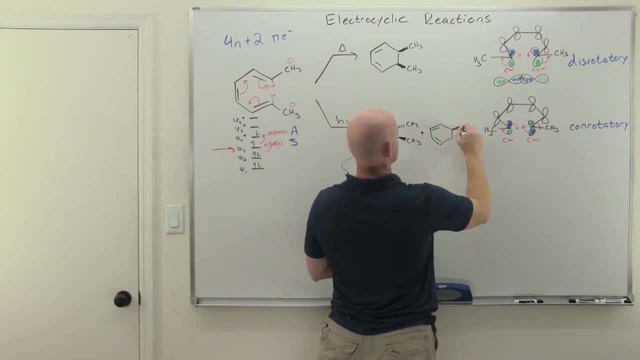 both enantiomers in this case, And so in this case I chose to have them both rotate clockwise, which put the blue shaded regions overlapping in the middle to form the new bond, But I could have had them both go counterclockwise. 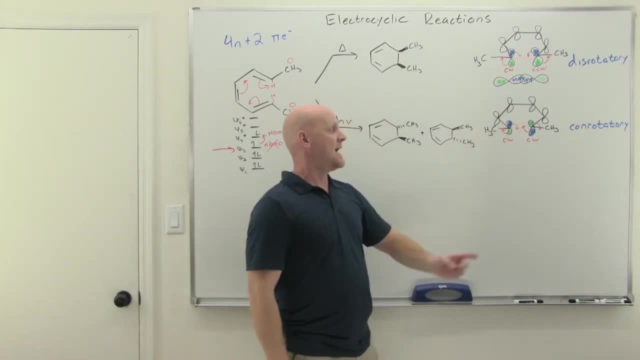 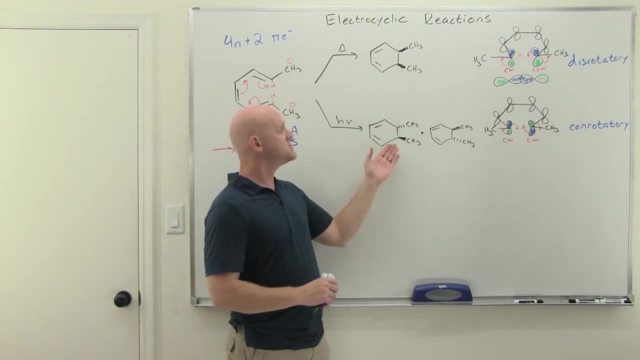 which would still be conrotatory, And it would have put the green regions out in the middle, And then two methyl groups would have ended up in exactly the opposite positions. And so that's why, if you do form a chiral compound, you do get the two enantiomeric versions of it. 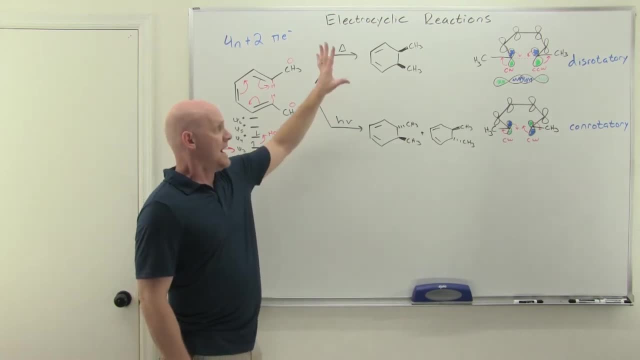 with these ring closures. Now, one thing to note, and I said it was important, when you're counting your pi electrons, to count the number moving in the transition state, not the number in your reactant, because these reactions are reversible. So if I was going to reverse this reaction, 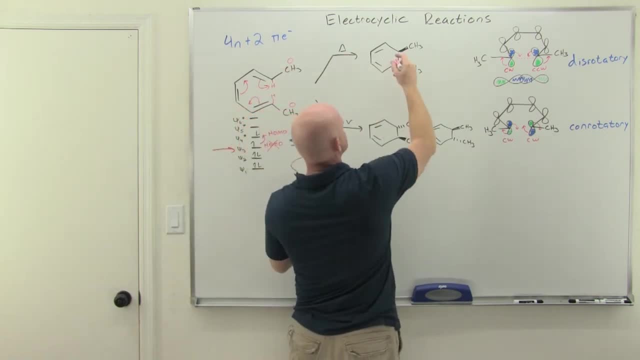 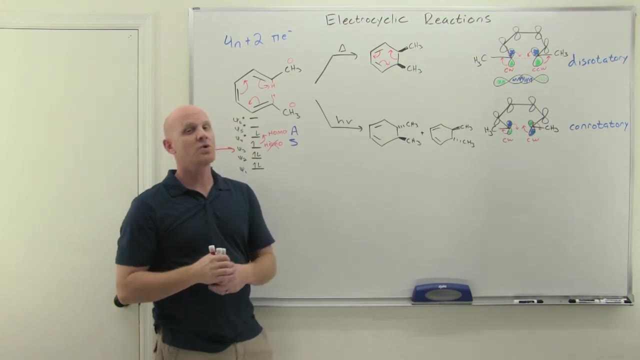 to go back to my open chain here. what I would do is just undo the arrows we did to close it, And so the mistake students will often make on a ring opening is they count their pi electrons and they're like oh 2,, 4 pi electrons. 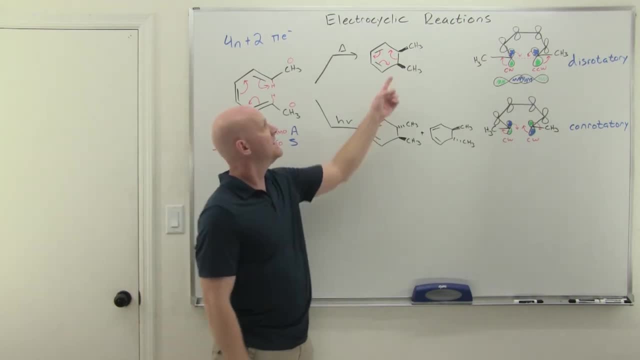 Great. Well, it's not again the number of pi electrons necessarily in the reactant, It's the number moving in the transition state, which is 2,, 4, 6.. That's the important part, And so, with it being 6 again, 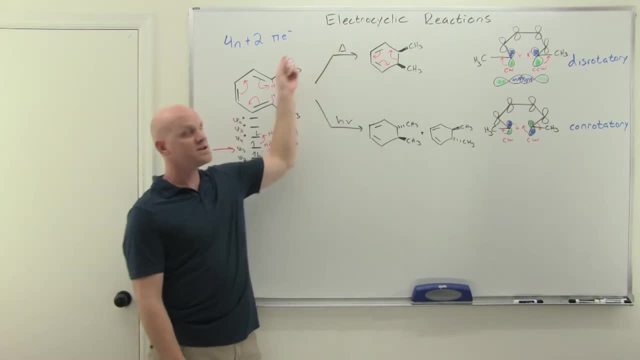 psi 3 would end up having been the homo under thermal conditions anyways, going back And again, just want to make sure you count your electrons correctly on a ring opening. The ring closure students don't have a problem with, but it's the ring opening that's tricky. 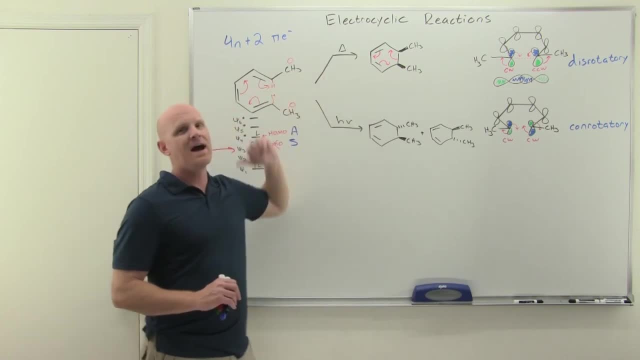 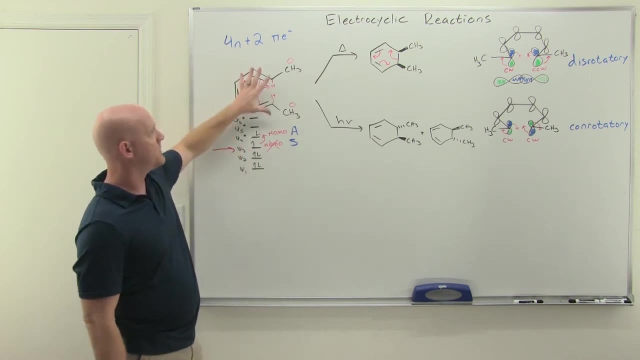 All right. So also, if you're doing a ring opening, I highly recommend you just do it backwards. So instead of doing the ring opening, do the ring closure, Do the reverse reaction. So pick your reactant. just pick randomly whether they're both out or one out. 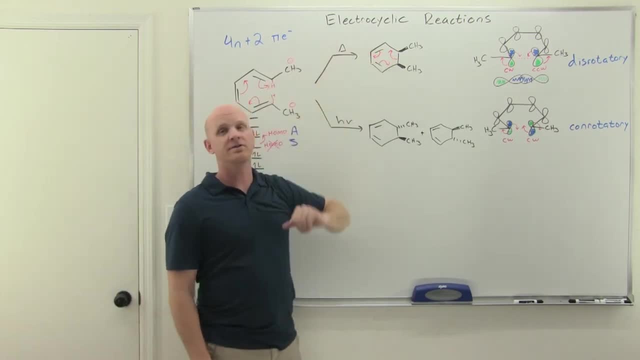 you're both in or one out, one in and then see if it leads to your product under your conditions, either thermal or photochemical. If it does, then you, by chance, got the right relationship, And if it doesn't, then you need to switch it. 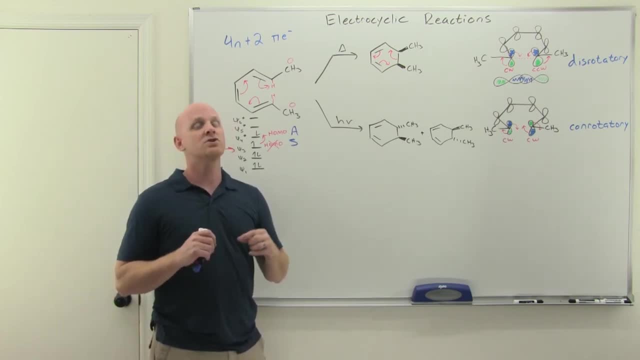 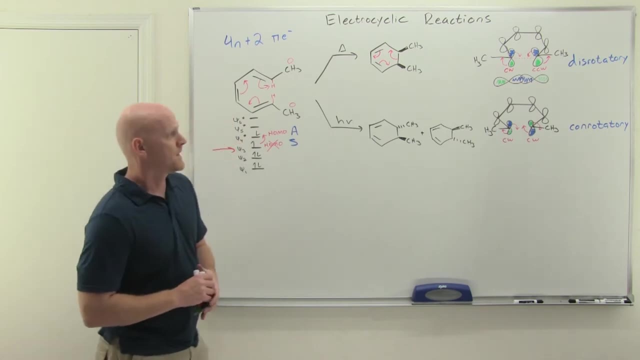 If you chose both out or both in and it works fantastic. If you chose both out and both in and it doesn't work, then you need to switch it to one out and one in instead. All right, So this again was a six pi electron transition state. 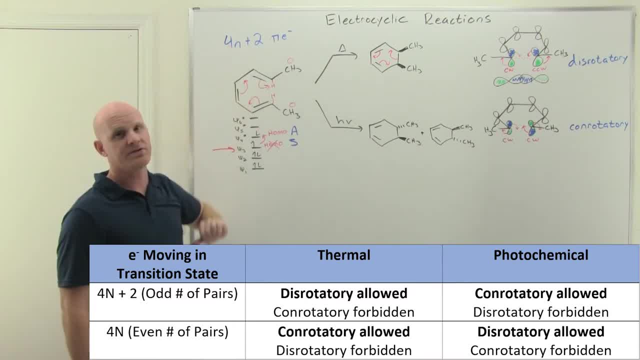 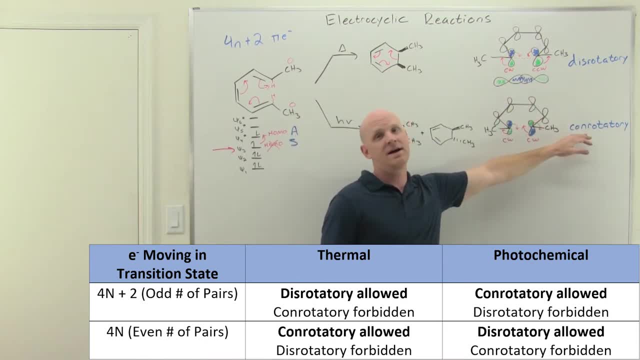 which is a four, n plus two number, And what we've now determined is that under thermal conditions, this rotatory is allowed, con rotatory forbidden. Under photochemical conditions, con rotatory is allowed and dis rotatory forbidden. Another generalization we could make is that 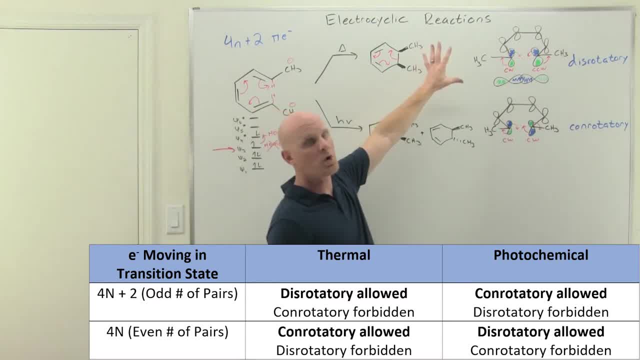 Psi three was symmetric and with a symmetric molecular orbital, it's dis rotatory that needs to happen, That's allowed. therefore con rotatory would be forbidden, Whereas in the photochemical conditions we were using Psi four star, which is anti-symmetric. 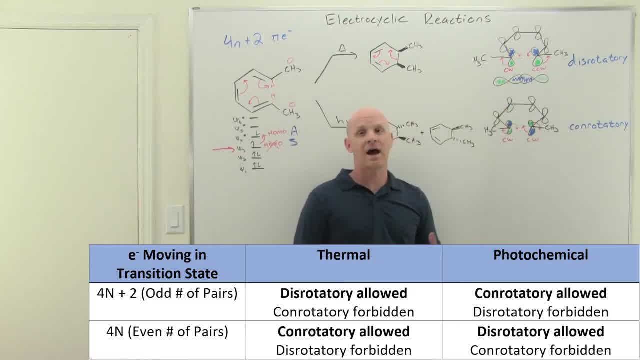 and for an anti-symmetric orbital, it is con rotatory that needs to happen and it's con rotatory that would be allowed. therefore, dis rotatory would be forbidden. Now, these generalizations we've made are for four n plus two pi electrons. 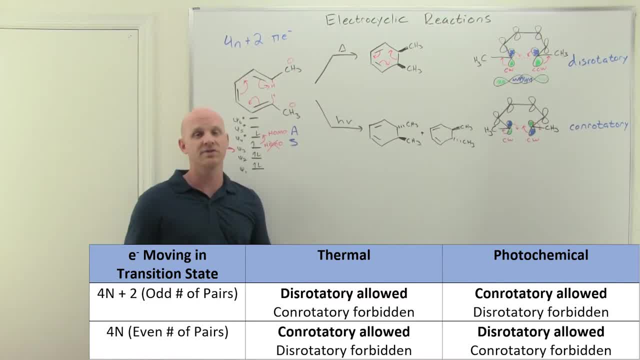 numbers like two electrons, six electrons, 10 electrons, If you recall, an odd number of pairs are the way to look at that. Cool When we do this in multiples of four, so a four n number of pi electrons, as we're about to here in a second. 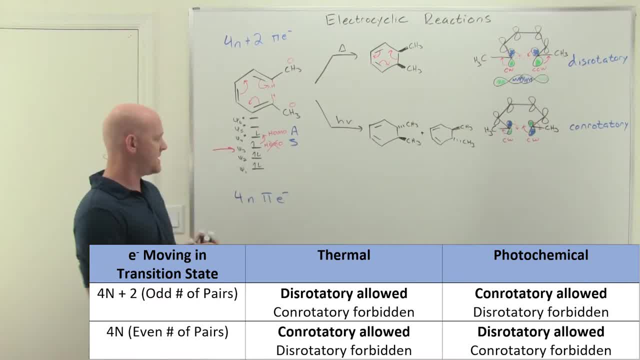 then it's all flipped. We'll find under that, you know, something where we're only moving a multiple of four pi electrons, an even number of pairs, that actually it's going to be dis rotatory. that is forbidden under thermal conditions. 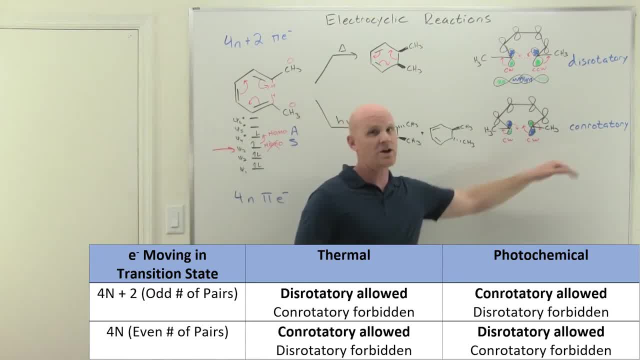 be con rotatory allowed And under photochemical it wouldn't be con rotatory allowed. it'd be dis rotatory that would be allowed and con rotatory forbidden. So it's all flipped when you're dealing with an even number of pairs of pi electrons. 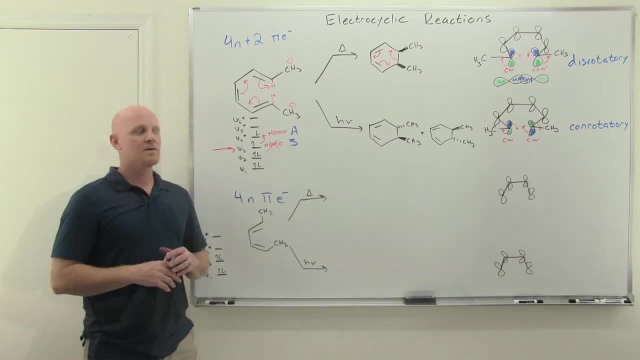 a multiple of four pi electrons. Let's take a look at an example. All right, in this next example here we're going to do another ring closure, But in this case it's only going to be involving the movement of four pi electrons. 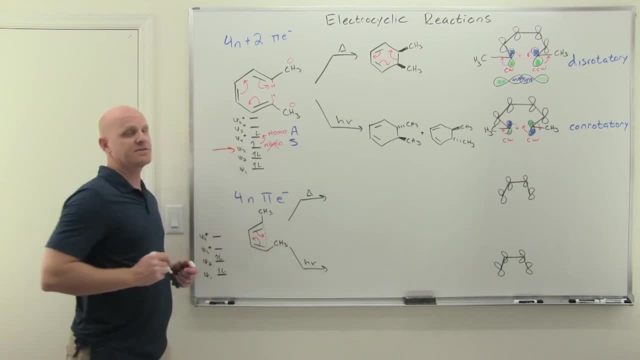 in the transition state, with only four pi electrons in our conjugated system. So in this case, then, it is psi two that is the highest occupied molecular orbital, And recall that psi one is symmetric, psi two is anti-symmetric, And if we do it under photochemical conditions, 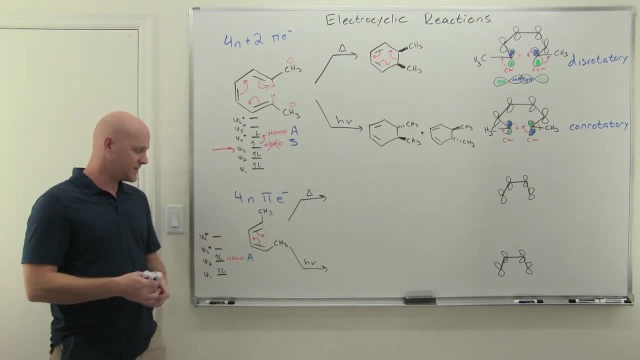 then we'd promote an electron. it'd be psi three star. That would be the new highest occupied molecular orbital, and it would end up being symmetric, as we'll see here in a minute. So let's go back to psi two, here being our homo. 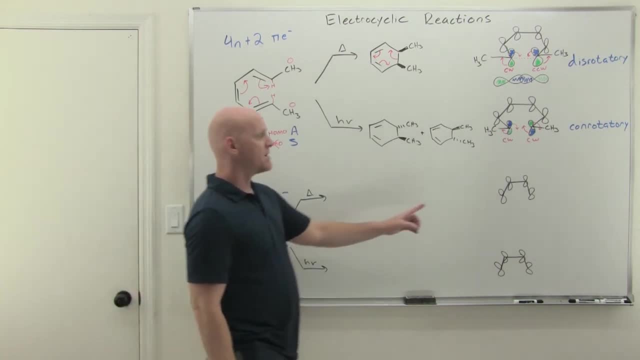 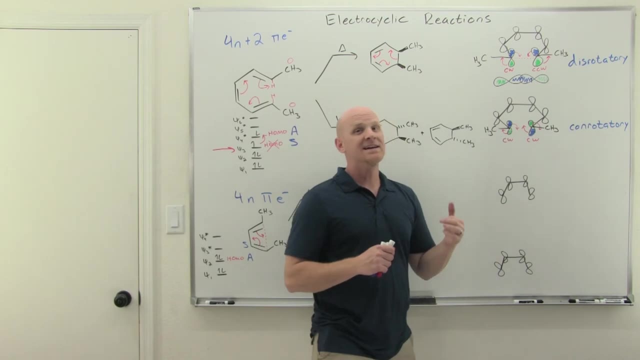 under thermal conditions And it's anti-symmetric. And again you could draw the entire psi two molecular orbital and it's on your study guide. However, the only part that matters for predicting stereochemistry in your product is just the ends here, where the new bond 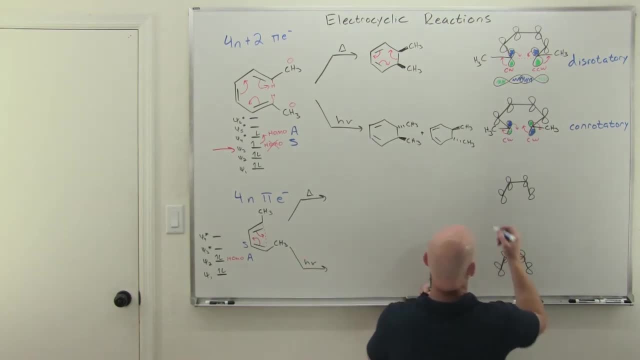 the new sigma bond, and so in this case, with it being anti-symmetric means the ends don't match. So when you've got an anti-symmetric molecular orbital, we learned that that's when conrotatory is allowed and disrotatory is forbidden. 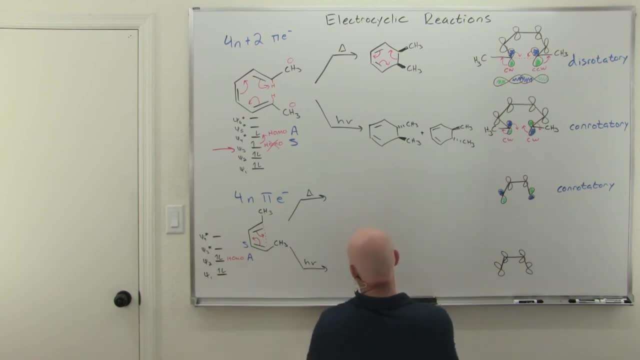 So before we rotate this, we could draw in where our methyl groups are. And if you look back on your reactant here, this methyl group is out. There's a hydrogen pointing in. This methyl group is in. There's a hydrin out over here. 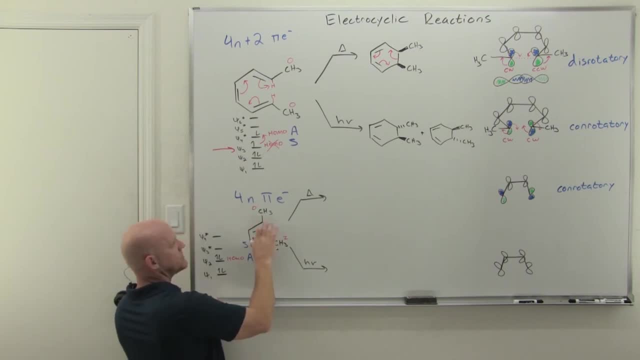 And so one methyl group is out, One methyl group is in. I only drew those hydrins in so we could make sure we knew what out and in meant. So but one's out, one's in, And a couple different ways you can look at this. 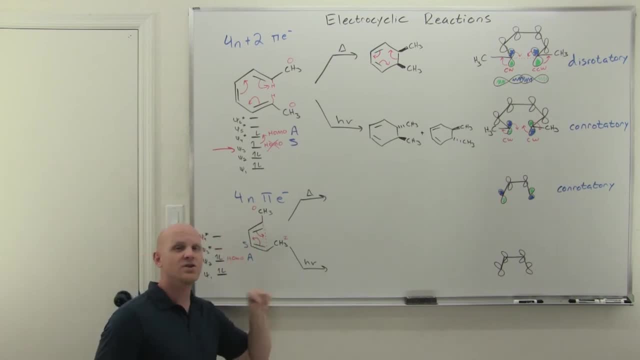 So one thing I do is I say: okay, one's out, one's in. What would Diels-Alder do with that? Well, Diels-Alder with one out and one in Diels-Alder would make them trans. 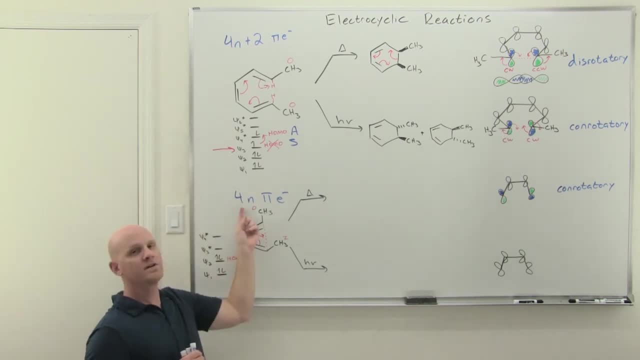 But Diels-Alder is for four n plus two pi electrons. We're dealing with four n pi electrons And so under thermal conditions we're gonna do opposite of what Diels-Alder would do, which happens under thermal conditions And then the exact opposite of that. 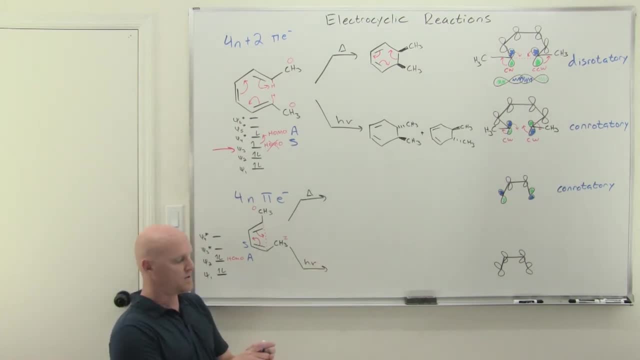 under photochemical conditions. And so one thing we could do without even looking at the molecular orbitals, we could just say, okay, well, we're gonna form a four-membered ring. So in this case, one out, one in. 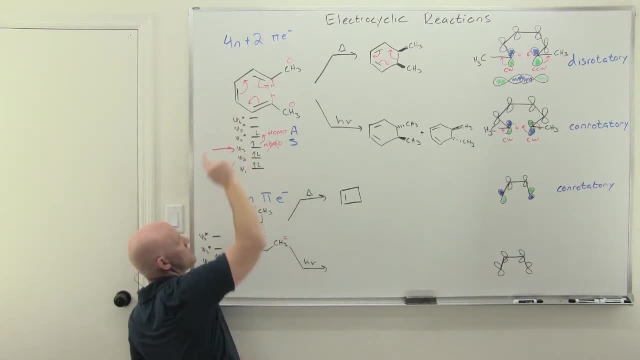 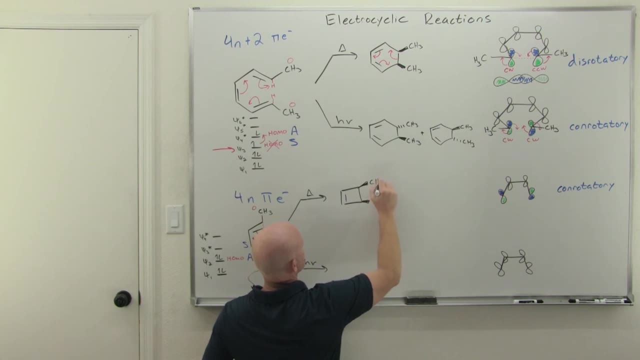 Diels-Alder would make them trans, but that's a four n plus two number of pi electrons. This is only a four n, And so we're gonna make them cis. Whether we make that both wedges or both dashes, it does not matter. 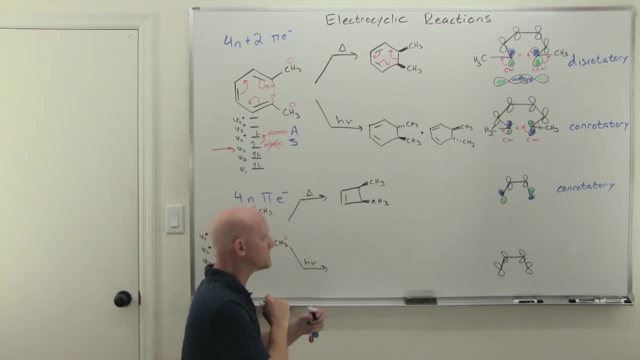 And it's a meso, And so instead of drawing two products, it's just the one meso compound again, whether you made them wedges or dashes. So you could predict that right off the bat. And if you do it under photochemical conditions, 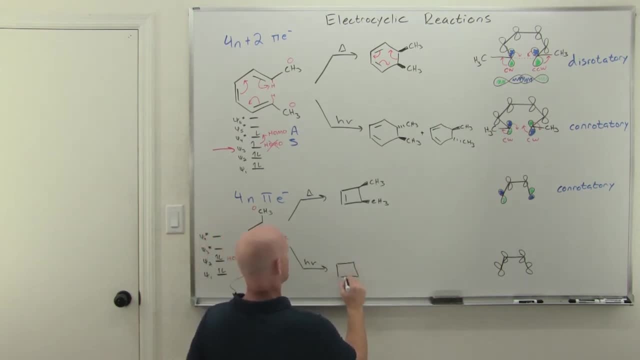 well then, it should be the opposite of that, And these should end up trans, And this is not a meso compound. So you're gonna get a pair of enantiomers, But I haven't really actually shown you how to predict these products. 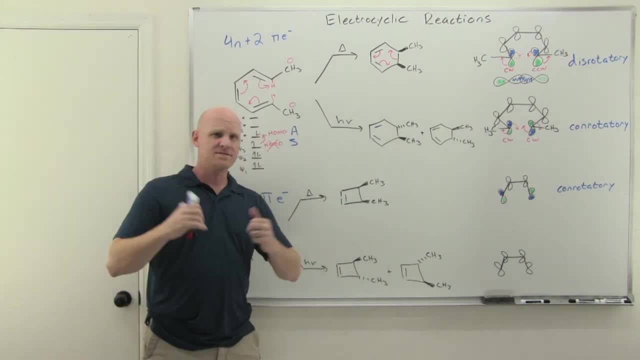 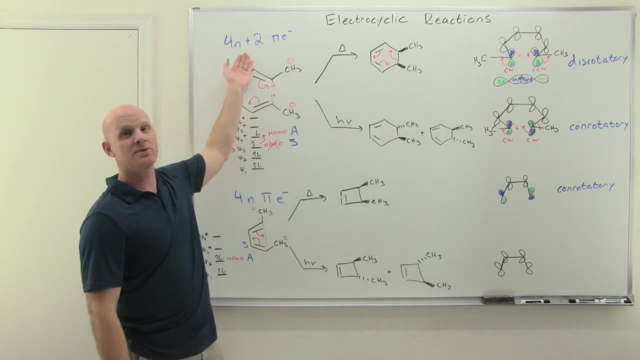 like from a conceptual standpoint. It's just memorizing some things and you know pattern recognition And we know what Diels-Alder does. and does it do the same as Diels-Alder? Well, if it's four n plus two pi electrons, 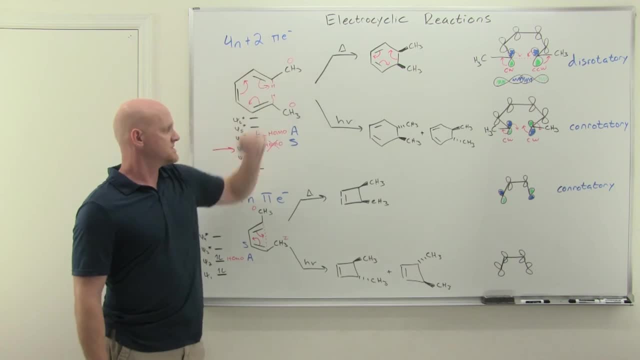 moving in the transition state, then yes, it does So, at least under thermal conditions. But if it's four n pi electrons, then under thermal conditions it would result in what's the opposite of the Diels-Alder. All right. 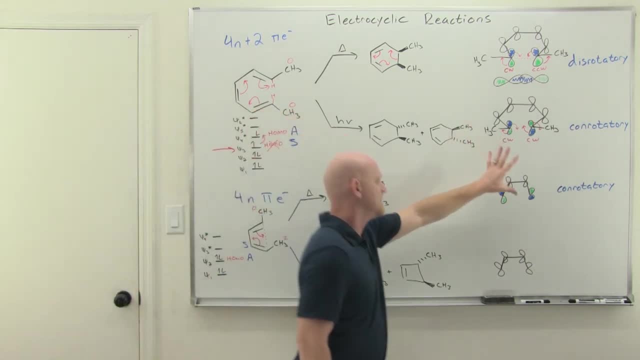 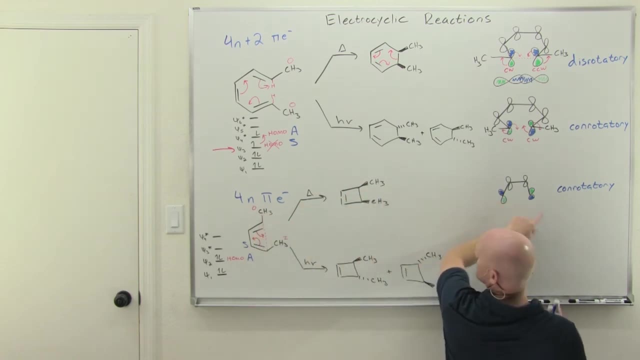 So again, that's just pattern recognition. But let's take a look again in our molecular orbital see what's really going on. And in this case again we've got the one. as we rotate this on the right is the methyl group pointing out. 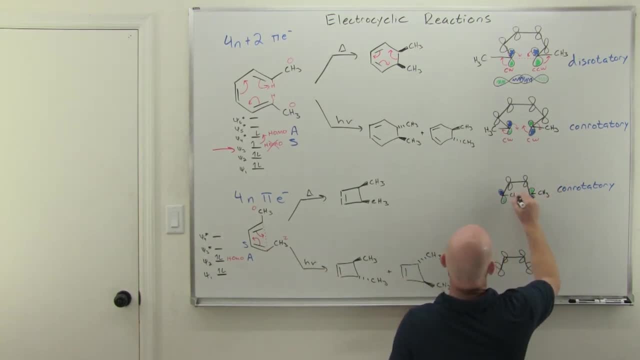 So, but the one on the left is gonna be the methyl group pointing in, So one's out, one's in, And now we'll see that it's gotta be conrotatory. But again, we memorized that. but we can see why that has to be here. 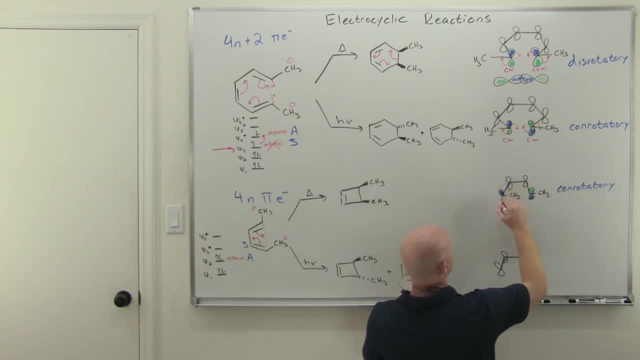 with this being anti-symmetric, And if I take the one on the left- and again I tend to make the one on the left first- go clockwise, Well, that's gonna put the blue group out in the middle where we're forming the new bond. 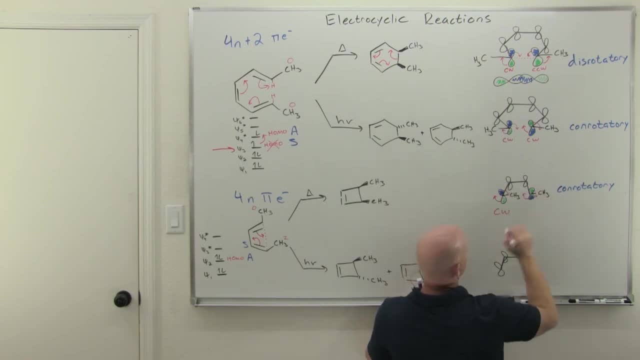 So to make sure the blue region on this one overlaps in the same region to get constructive overlap in phase overlap. So I can see that this one also needs to go clockwise, because they're going in the same direction both clockwise or both counterclockwise. 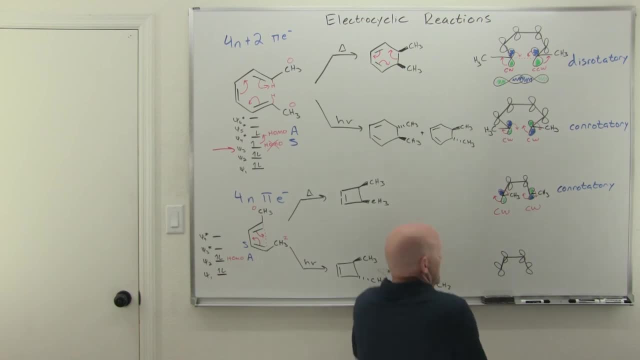 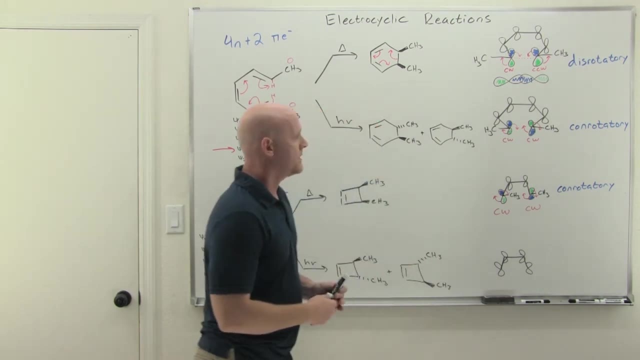 That's again what conrotatory means, And once again, that was just a generalization. we made too that with an anti-symmetric orbital the only way you get constructive overlap is with conrotatory rotation here. So cool, If you notice what happens then too. 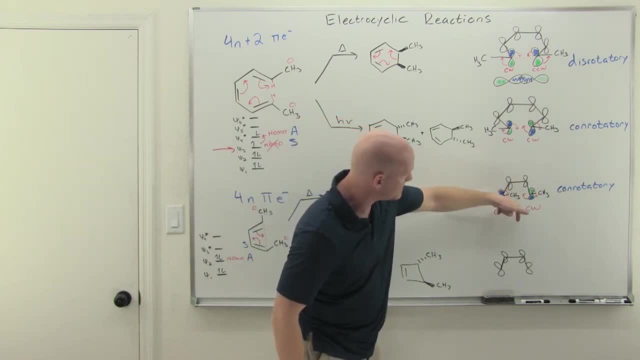 is that the methyl group here on the left is gonna get forced down and be a dash. The one on the right also is gonna get forced down and be a dash, And so they're gonna both end up cis to each other as dashes. 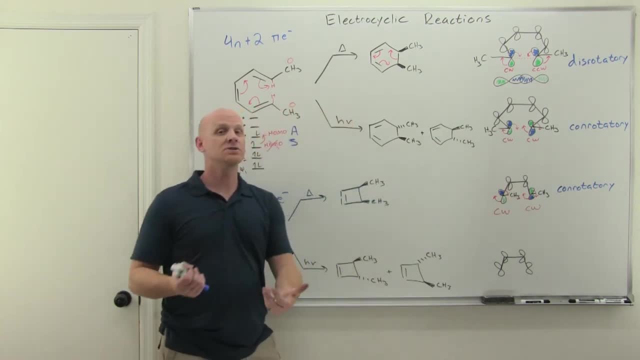 So, but again, I chose clockwise and clockwise. Had I chose counterclockwise and counterclockwise, then it'd be the opposite and both methyl groups would have been forced up. The key is: is they're gonna end up cis? 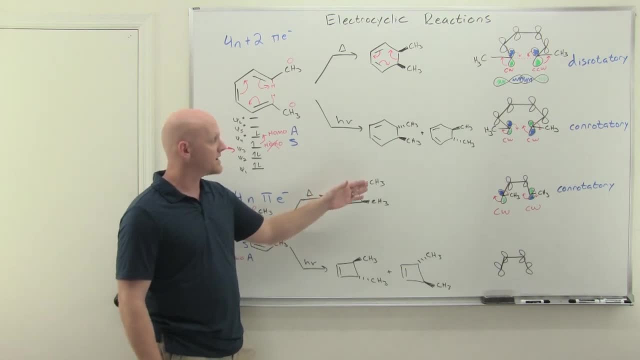 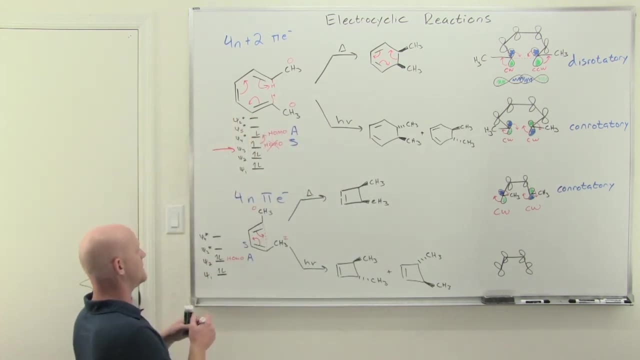 And in this example that's a meso compound, So it didn't matter whether again I made it both wedges or both dashes Now in the other example here. so now once again, we are gonna promote an electron under photochemical conditions. 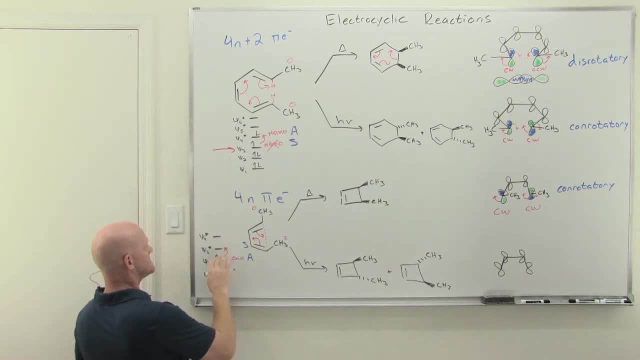 From Psi two up to Psi three, And so Psi two is no longer the highest occupied molecular orbital. It's now Psi three, under photochemical conditions, and it's symmetric. And if it's symmetric it means the ends of the molecular orbital match. 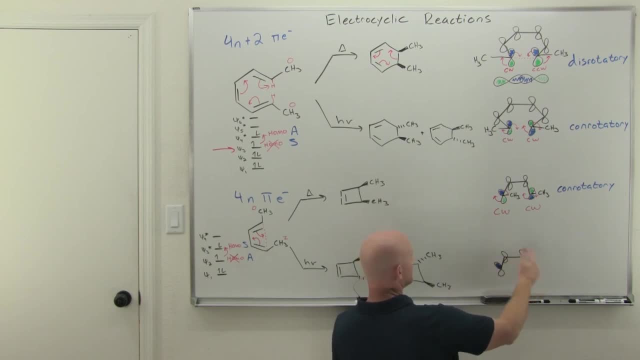 And again, you can draw the whole thing and you might be on the hook for doing so on a test or something. It's on your study guide, but I'm not gonna do it here Again. my point here is just to predict that it's gonna match. 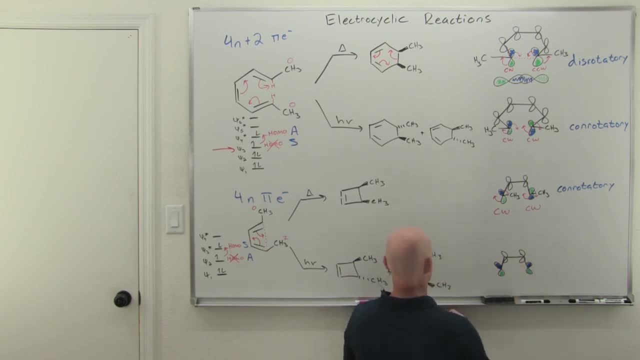 I'm not gonna predict stereochemistry but, like I said, the whole thing is on your study guide And once again so the one on the right. as we rotate, this is gonna point out the methyl group on the right, But the methyl group on the carbon on the left. 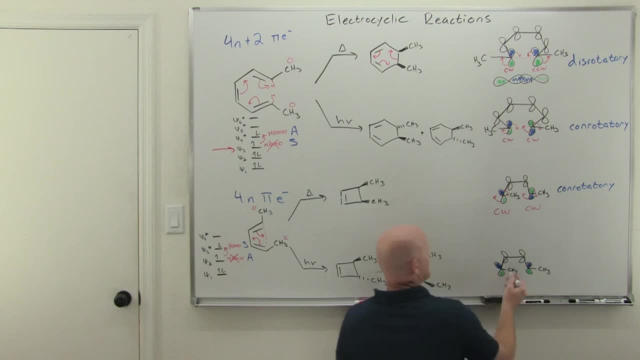 is gonna point in. Well, with a symmetric molecular orbital it's gonna have to be dis-rotatory to get constructive overlap. So we say that dis-rotatory will be allowed, which means con-rotatory would be forbidden, And once again, 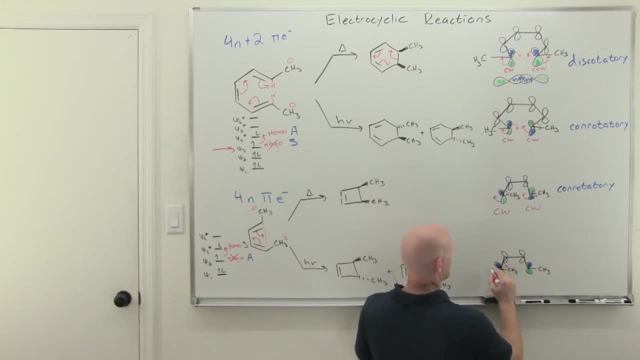 I'm gonna rotate the one on the left clockwise And that's gonna be the same And that's gonna cause this methyl group to go down. It's gonna put the blue region in the middle And to get constructive overlap then on the other side. 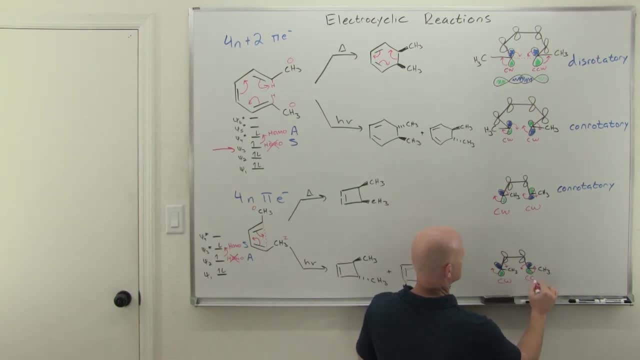 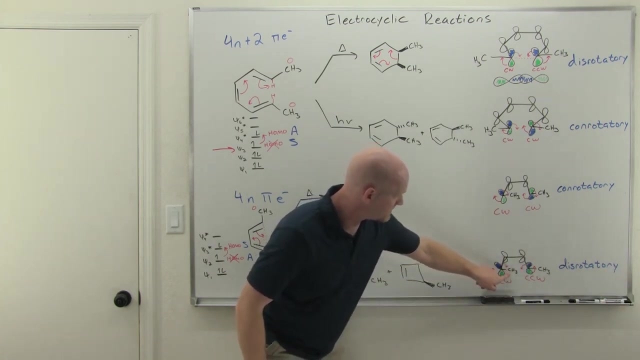 I'd have to rotate counterclockwise, And with one clockwise, one counterclockwise again. that's why dis-rotatory is allowed. Cool, We can also see that one methyl group is gonna be forced down and be a dash. 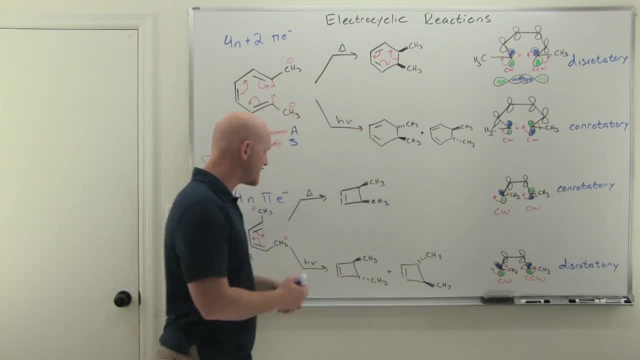 The other one's gonna be forced up and be a wedge. They're gonna be trans to each other in the product And again I chose clockwise and counterclockwise. I could have chose counterclockwise and clockwise And that's why you get both enantiomers in this case. 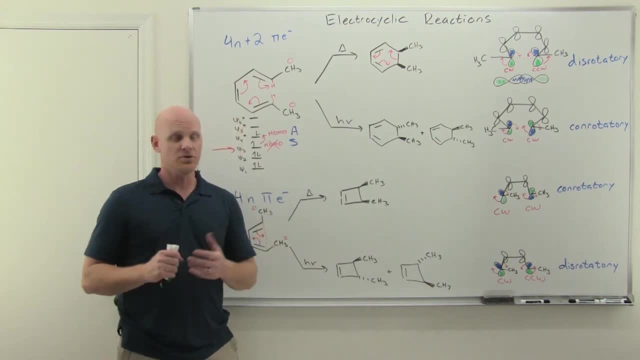 Cool. So we've got a couple of different ways of predicting products. If you know your Diels-Alder real well, all your cycloadditions and your electrocyclics based on the number of pi electrons moving in the transition state. 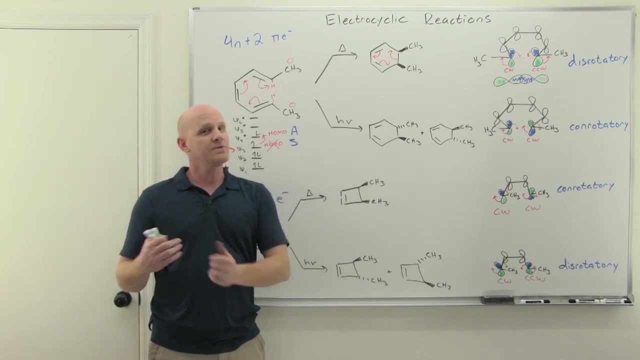 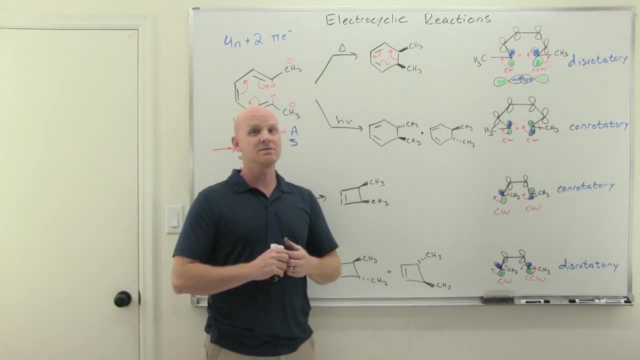 you can actually compare them to what you know about Diels-Alder, which a lot of students do. However, if you draw in your molecular orbitals involved, whether it be cycloaddition or electrocyclic, you can figure out just by looking. 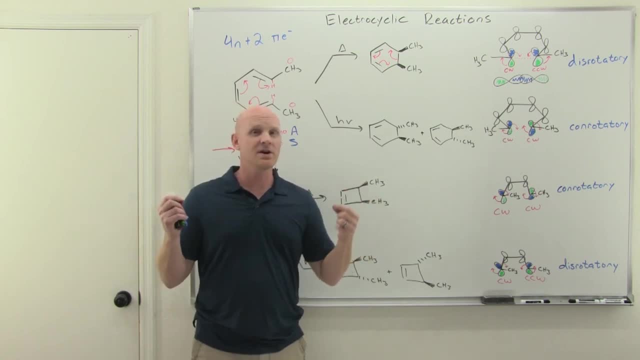 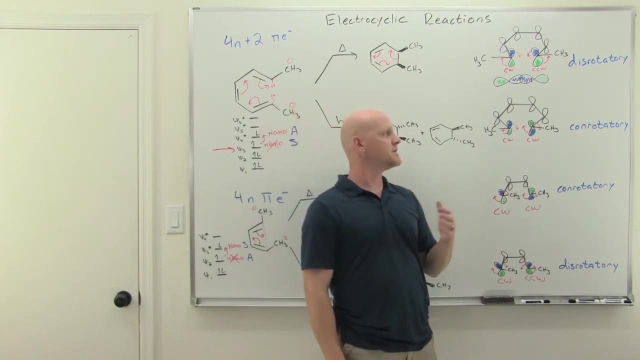 Whether your molecular orbital's symmetric or anti-symmetric. you can figure out whether you need disrotatory motion for constructive overlap to occur, in which case disrotatory would be allowed and conrotatory forbidden, Or if it's the opposite, because you have an anti-symmetric molecular orbital. 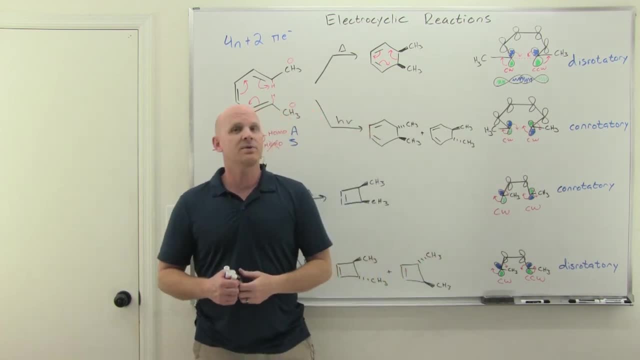 then conrotatory would be allowed and disrotatory forbidden. Similar things with figuring out whether it's superfacial, superfacial or superfacial and terafacial. back with the cycloadditions. But this is kind of the deal. 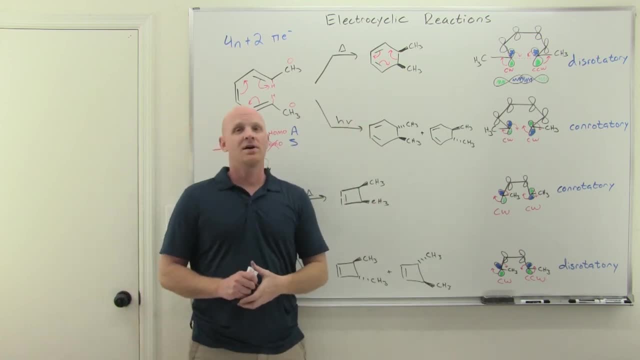 Hopefully you've got a much better grasp on these electrocyclic reactions than you did 10 minutes ago. Thank you,